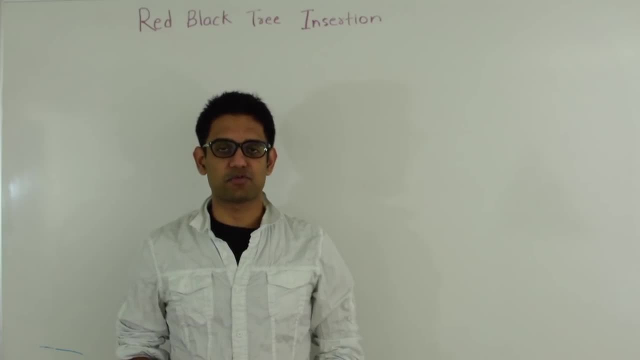 The time. complexity for red-black tree operations is similar to AVL tree, but the balancing condition in red-black tree is less restrictive, which is why we have less rotations, which is why red-black tree is more preferred than AVL tree. Examples of red-black tree is like tree map or sorted map in Java. 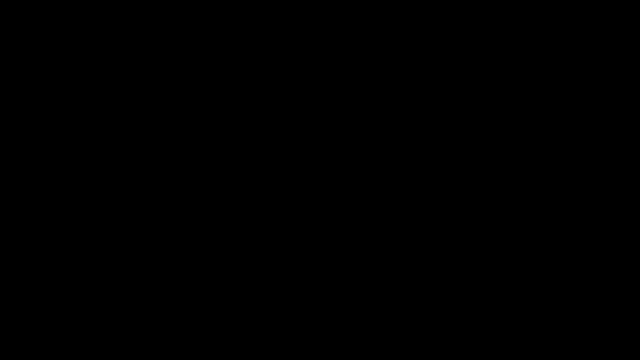 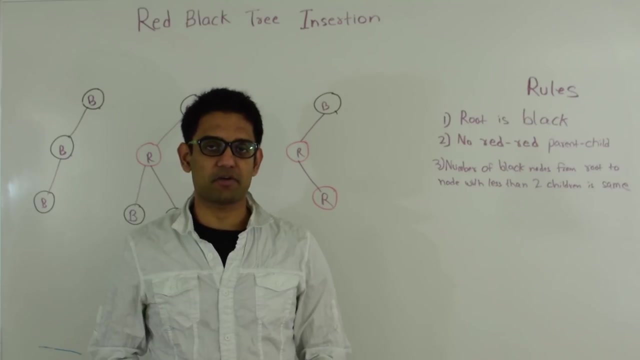 So next let's try to understand the rules of red-black tree. First of all, red-black tree is a binary search tree, So if a tree does not follow the properties of binary search tree, it cannot be a red-black tree. After that, the nodes of red-black tree are either black or red. 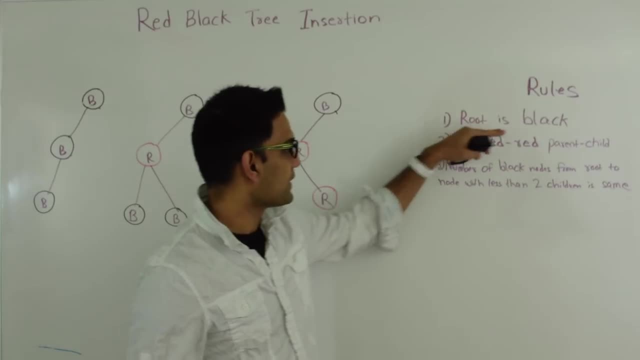 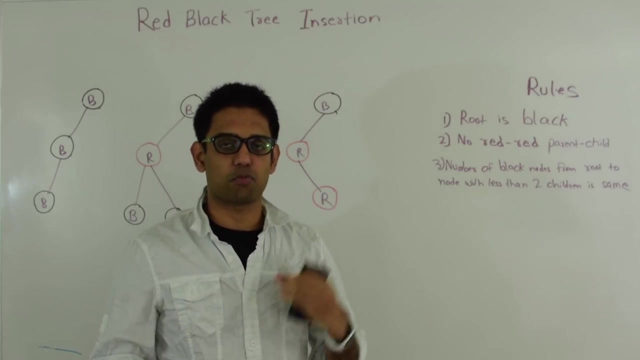 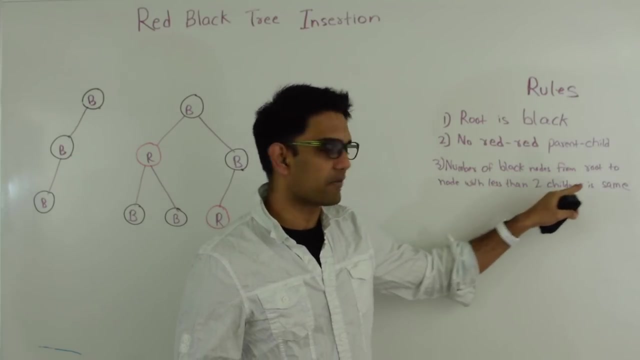 So these are the three conditions of red-black tree. The root is always black node. There is no red-red parent-child relationship. Basically, both parent and child can live together. They cannot be red. One of them needs to be black, And then number of black nodes from root to node with less than two children should be same. 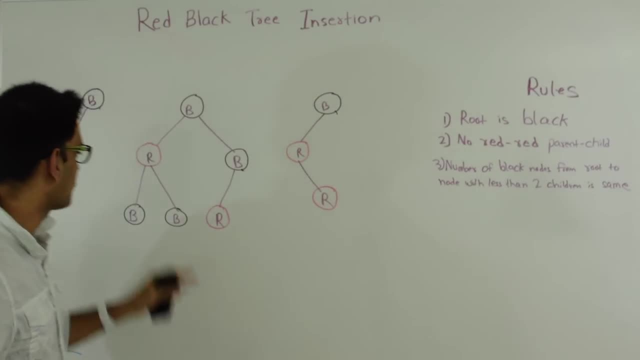 So let's understand these three conditions with the help of three examples here. So let's start with this one. First of all, let's find the nodes with only one child, So this and this node, and let's put a null there, So null and null. 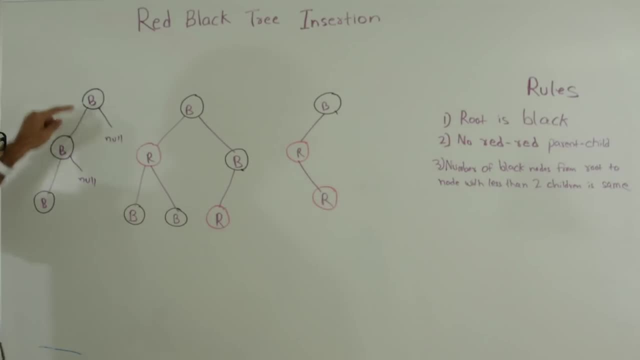 Now let's try to apply these three conditions: Root is black, So root is black. No red-red parent-child relationship. There is no red-red parent-child relationship. Number of black nodes should be same from root to nodes. So for this guy, root to this guy, it has onein this path it has one black node. 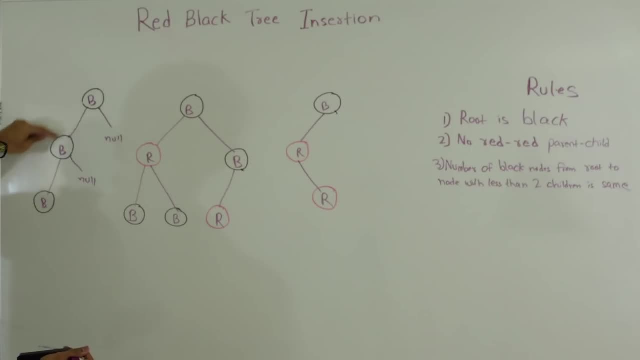 In this path here it has two black nodes. In this path here it has three black nodes. So it does not satisfy the rule number three. So this is not a red-black tree. Let's move on to this example. First, let's add a null node for a node which has only one child. 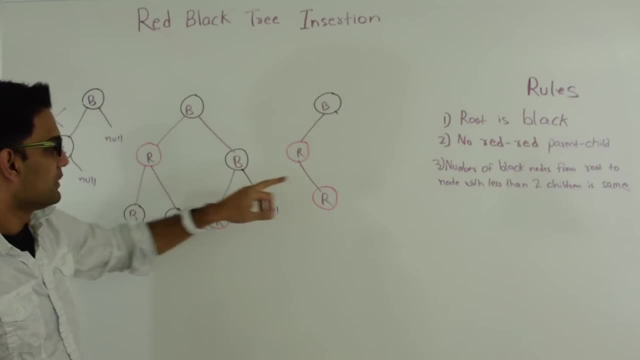 Now root is black. No red-red parent-child relationship. And let's count the number of black nodes in every path. In this path here, number of black nodes is two. In this path here, number of black nodes is two. In this path: here, number of black nodes is two. 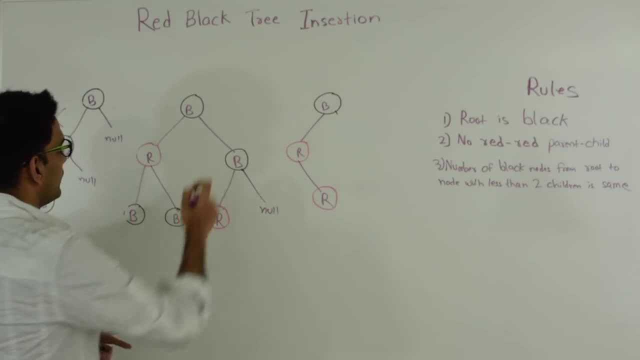 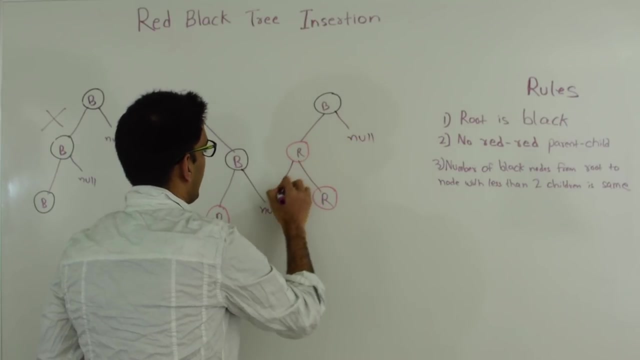 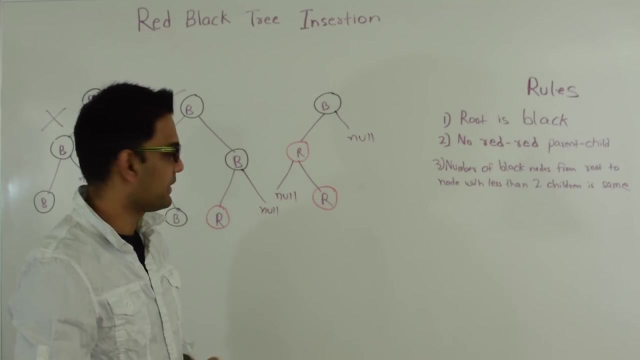 And in this path here number of black nodes is also two. So this is a red-black tree. So this is a red-black tree. Let's do for this one. So let's add null here. first, Root is black. Here we have this parent-child red-red relationship. 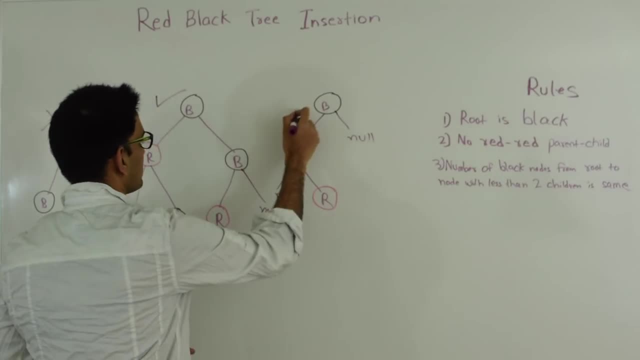 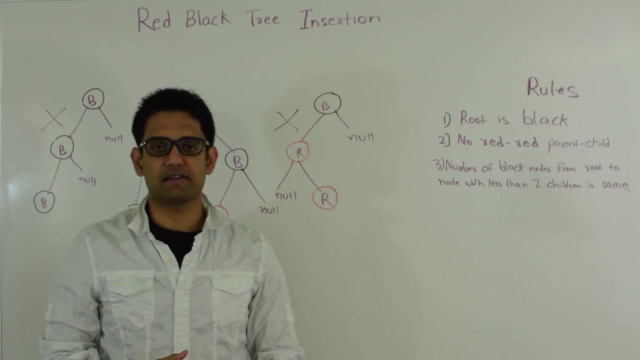 It means that it doesn't satisfy property number two, So this is not a red-black tree. Hopefully this helps you understand how the properties of red-black tree work. In the next section let's see the rules for insertion into the red-black tree. 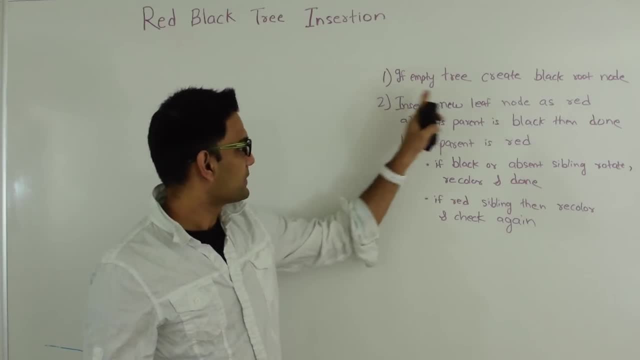 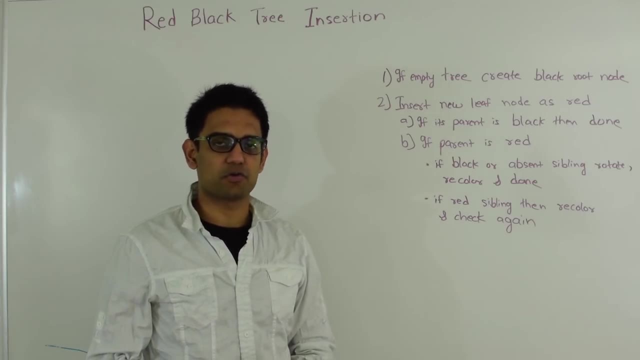 These are the rules for insertion into red-black tree. If the tree is empty, then just create black root node. If the tree is not empty, then the newly created leaf node should be red node. If the parent of this newly created leaf node is black, then we are done. 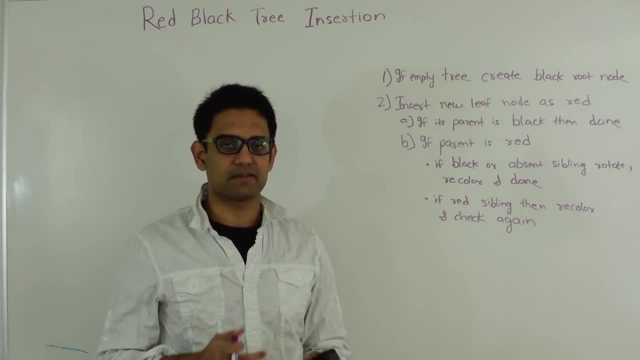 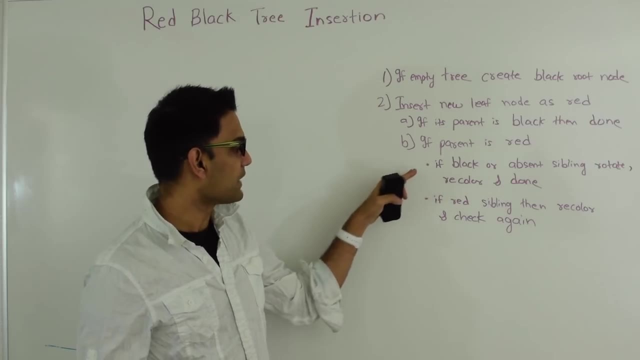 If the parent of this newly created leaf node is red, then we have that red-red conflict, red-red parent-child relationship. In that case, we have to do either this or this. So let's try to understand all these rules with the help of an example. 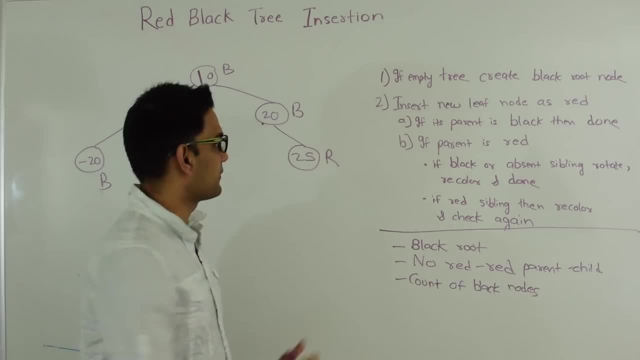 Creating a black root node for an empty tree is pretty trivial, so I'm not going to show that. So let's see, when I insert a new leaf node as red and its parent is black, what happens. So here I have a red-black tree. Let's make sure it's a red-black tree. 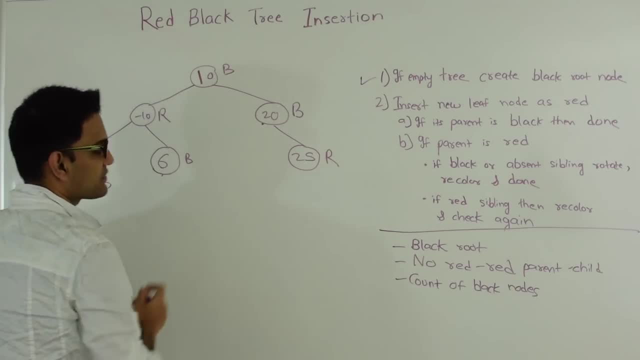 The root is black, There is no red-red parent-child relationship And the count of black nodes in all the paths is same. So we have four paths here. This one: The count of black nodes. The count of black nodes is two. 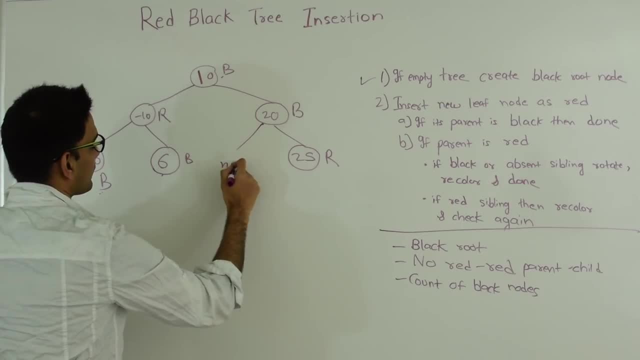 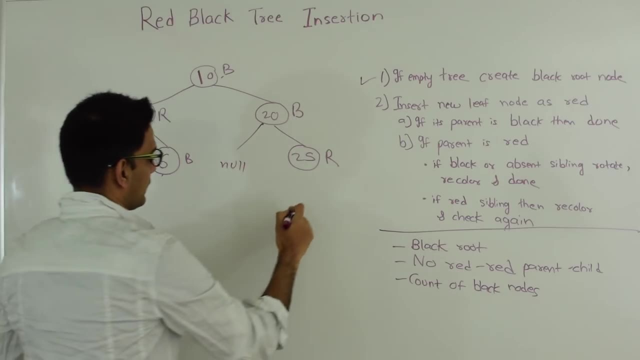 This The count of black nodes is two. We add a null here. This The count of black nodes is two And this The count of black nodes is two. So this is indeed a red-black tree. Let's try to add four into this red-black tree. 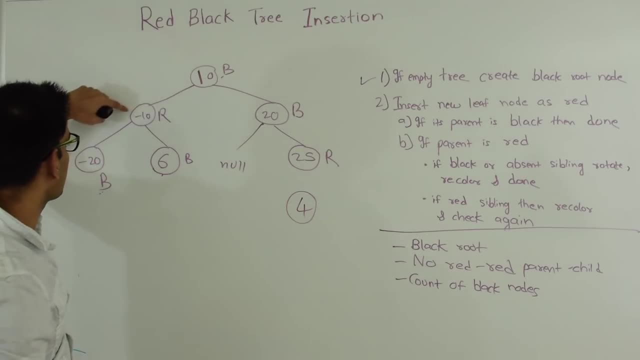 So we go to root. Four is less than ten, So we go on the left side. Four is greater than minus ten, So we go on the right side. Four is less than six, So we go on the left side And create a new red node. 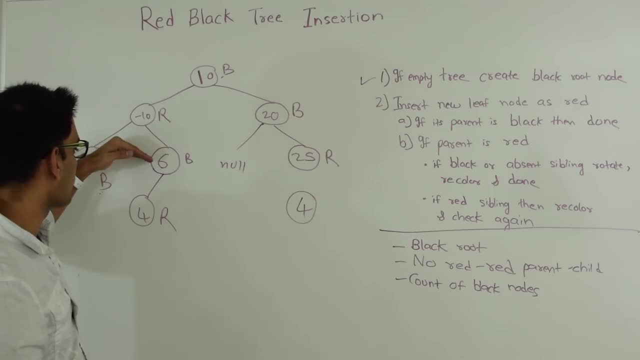 Now adding this, Since the parent of this Red node is black, adding this red node did not violate any of the three conditions. Our root continues to be black node. No red-red parent-child relationship is created because this guy's parent is black. 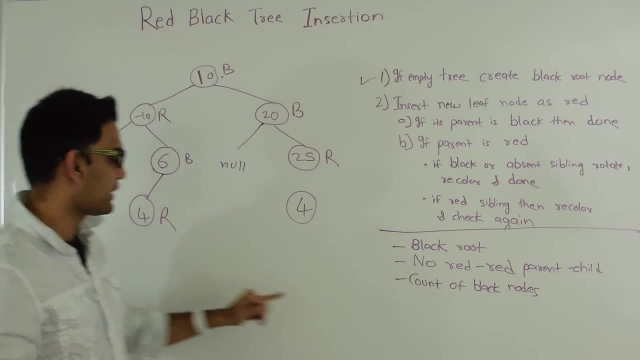 And since the newly created node is red node, it did not affect the count of black nodes. So if the parent is, If the parent is black, then it's a trivial case. So let's see what happens if the parent is red. 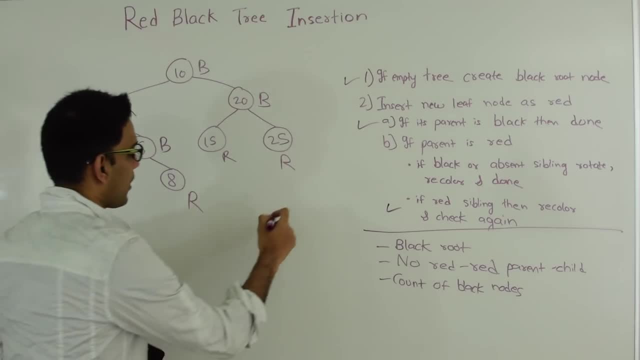 Here I have another red-black tree And now I'm trying to insert four into this red-black tree. So four is less than ten. We go on the left side: Four is greater than minus ten. We go on right: Four is less than six. 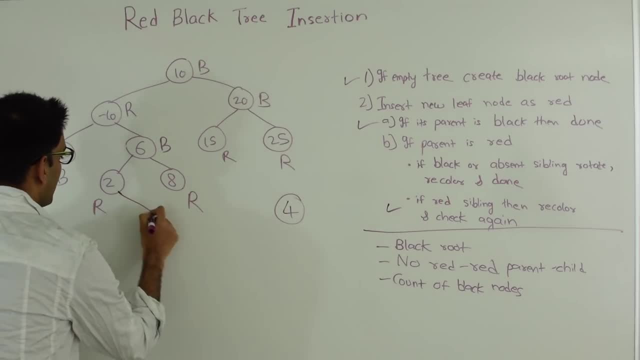 We go on left And then four is greater than two. So we go on the right and create four, And the color of newly created leaf node is always red, But the parent- The color of its parent- is also red, which means that we violated this condition too. 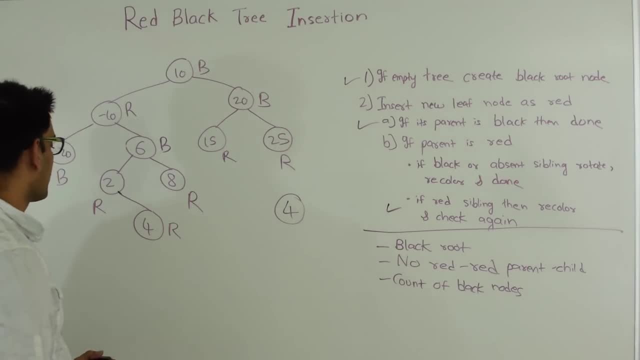 where parent-child relationship should not be red-red. So what do we do in this situation? What we do is we look at the color of its sibling. So we're going to look at the color of parent's sibling, which is eight, And the color of eight is red. 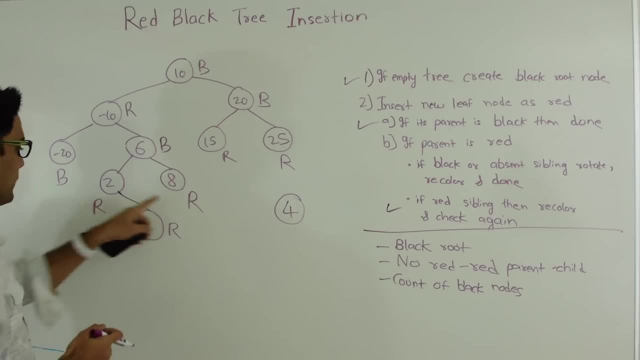 So we are in this condition here: If the sibling is red, then you have to do some recoloring, and then you have to recheck at the above level. So what we're going to do is We're going to change the color of 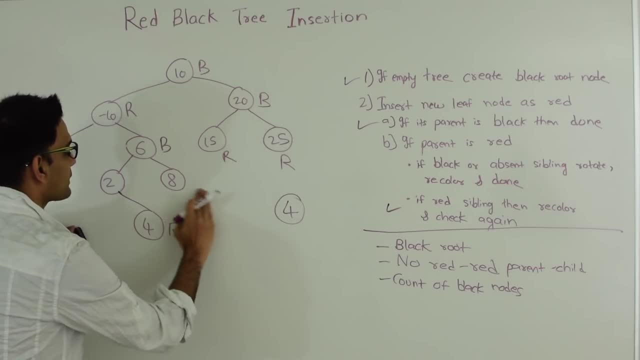 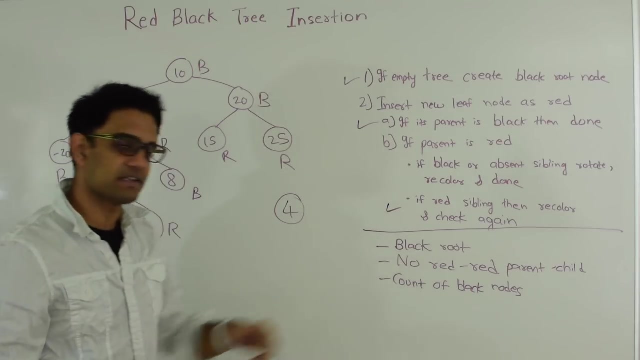 This guy and this guy to be black, And if the parent is not root, then change its color to be red. So what happened here was we broke this red-red relationship and converted into black-red relationship, And we also did not change the count of the black nodes, because the black node was here. 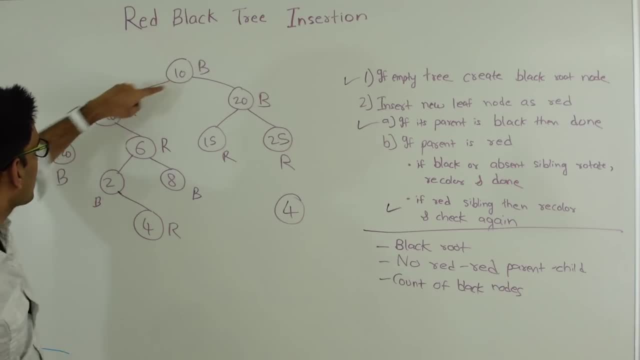 and we just pushed it down. So the count of the black node in all the path continues to be two. But since we did that, we created this red-red parent-child relationship here. Now to break this red-red parent-child relationship, we're going to look at minus tenth sibling, which is twenty, and color of twenty. 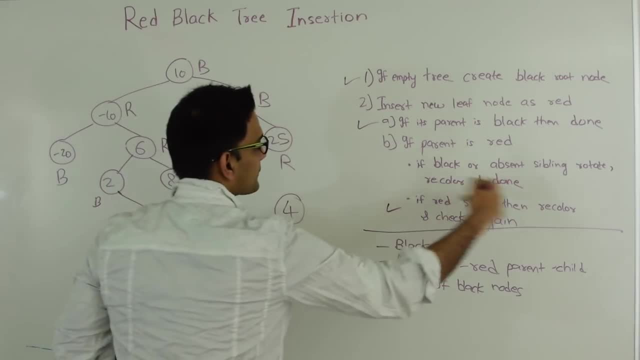 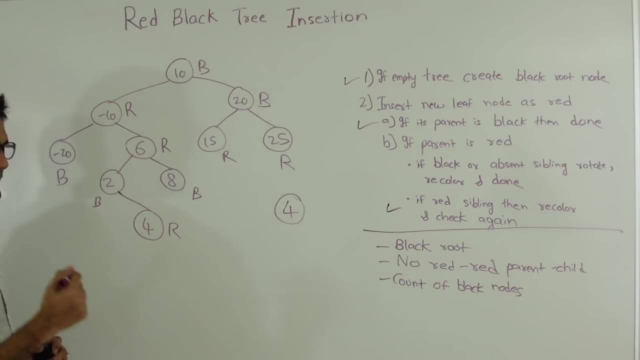 Color of twenty is black. So we'll have this condition and we'll look at it little later. We have one more condition to check: What if this guy was root? And let's see that example. Here I have same tree as before. 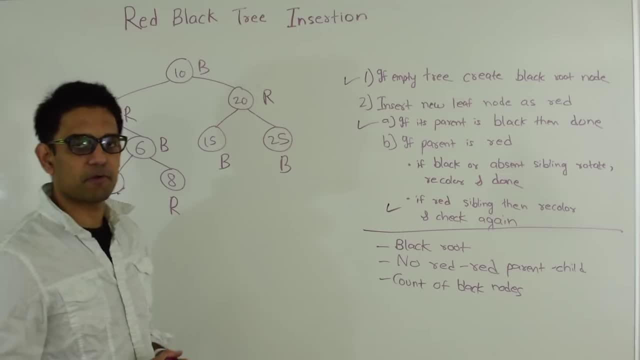 The only thing changed is I changed the color of this node to be red before it was black, And I changed the color of these nodes to be black before they were red. So now we'll again try to insert four. So four is less than ten. 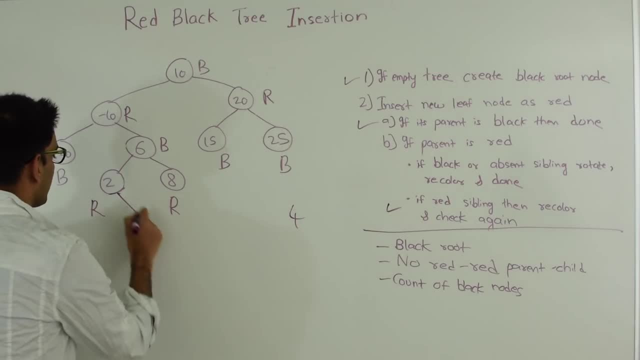 It's greater than minus ten, It's less than six, It's greater than two. So four gets inserted here And color of four is red. So this created this red-red relationship. We looked at two siblings, which was red. To break this red-red relationship, we changed the color of this and this to be black. 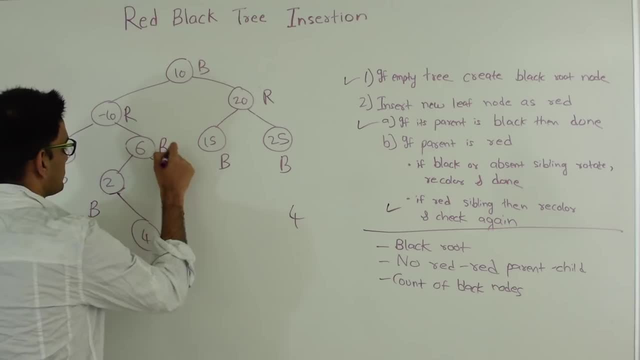 And changed the color of this to be red. So this solved the red-red relationship here, But it created new red-red relationship here. So we again looked at this guy's sibling and this guy was red. So again we changed the color of this to be black. 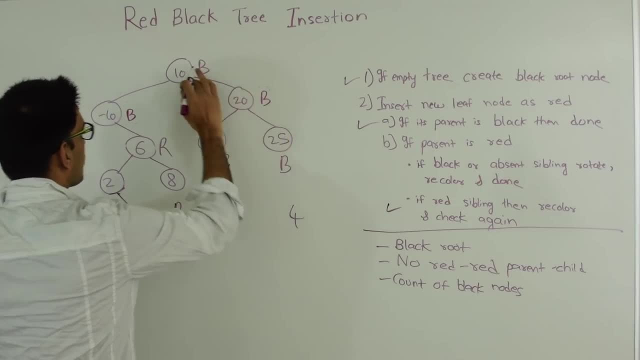 And this to be black. And now we go to that parent. If this parent was not a root node, Then we would have changed its color to red And then we would have checked with its parent. But in this case the parent is root node. 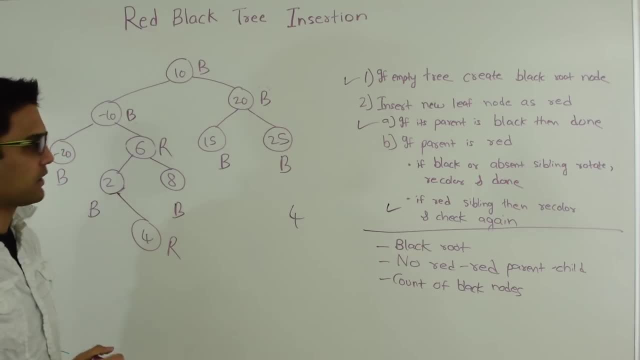 Which means that you stop and you do not change the color of black node And we do not change the color of root node. So then, this is now a red-black tree. Its root is black, There is no red-red relationship, And the count of black nodes in every path is same. 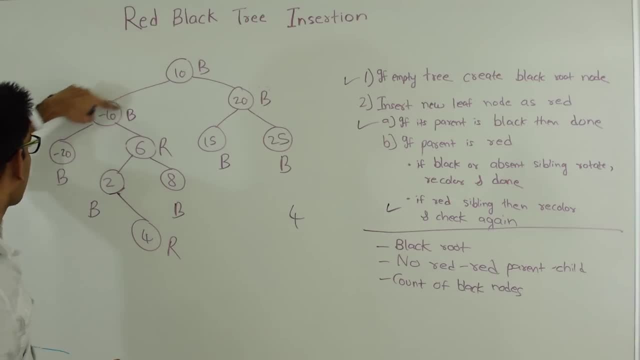 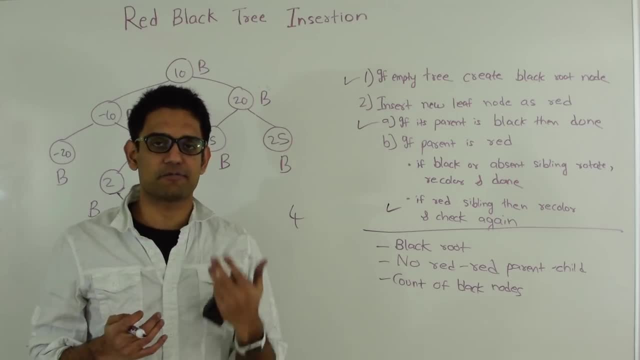 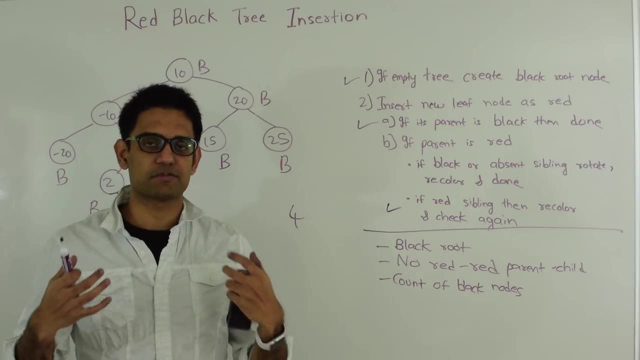 So to summarize: If the sibling, If the node at which red-red relationship is happening, We check its sibling. If the sibling is red, We recolor both this siblings to black And change that parent to red Only if that parent is not a root node. 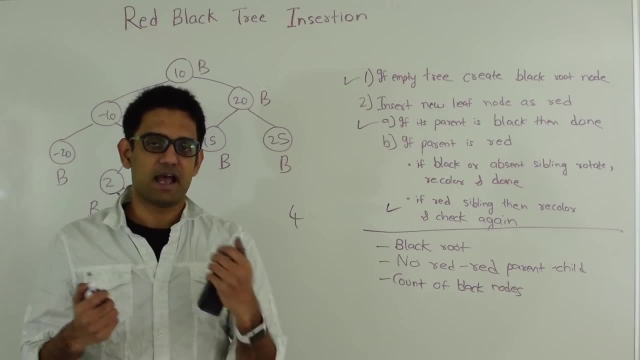 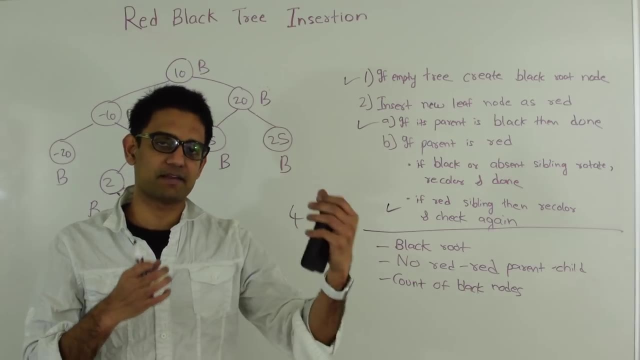 If it is root node, Then we leave as it is, And if we change the parent to To red, Then we recursively check if it is not creating a red-red relationship with its parent, And if it is, then we keep fixing this recursively. 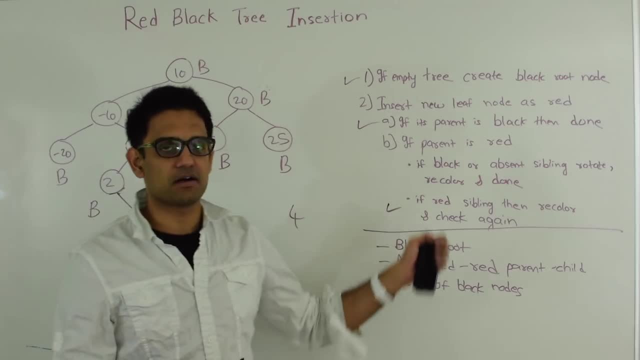 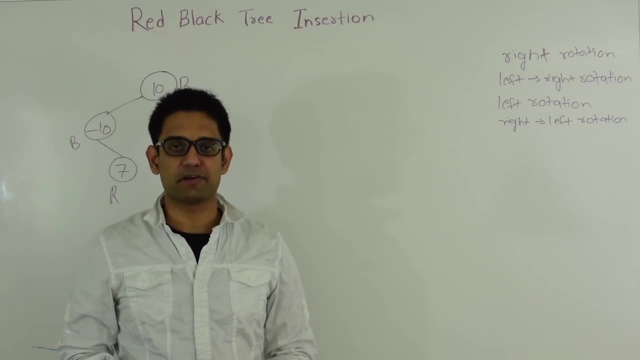 So next Let's see what happens if the sibling is black or if the sibling is absent. We have two more conditions to look at What happens if the sibling of the node at which red-red conflict is happening is black or absent. In either of the case, we will do one of the four things. 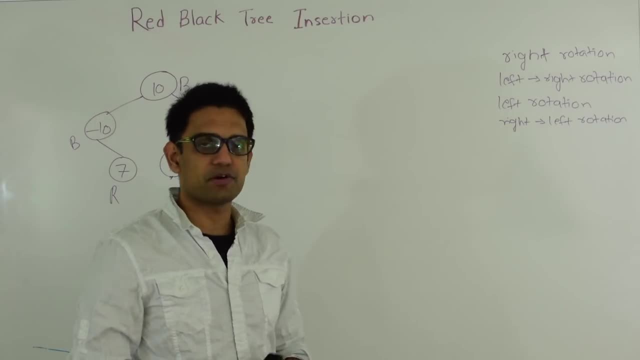 Right rotation, Left, followed by right rotation, Left rotation or right rotation, Right rotation, Right rotation followed by left rotation. If you remember AVL tree, We did similar rotations to bring to balance the AVL tree, So let's try to insert 13 in this red-black tree here. 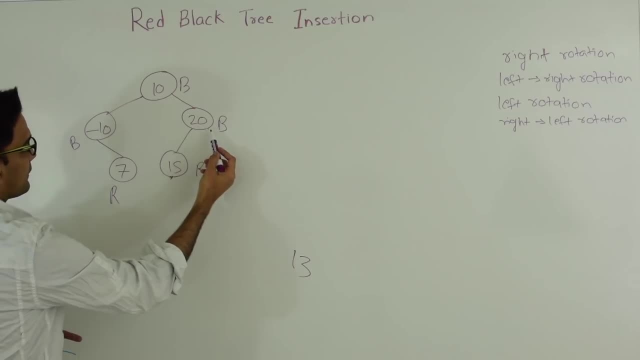 So we go to the. 13 is greater than 10.. So we go to 20.. 13 is less than 20.. So we go to 15.. 13 is less than 15.. So we add 13 right here. 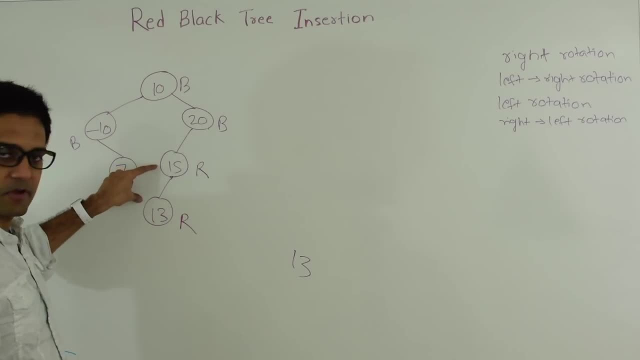 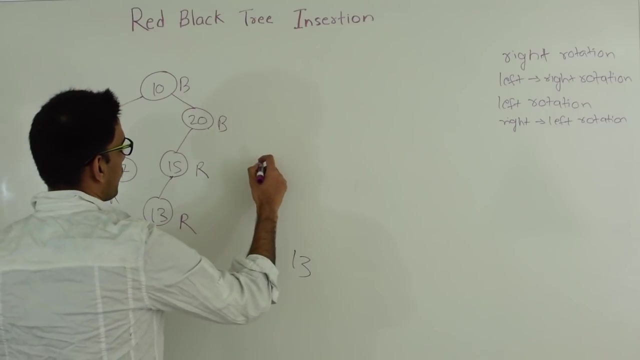 And color of 13 is red. So at this point of time, we have red-red conflict Here. we look at its sibling. The sibling is missing. So what we are going to do is we are going to do a rotation at this point. 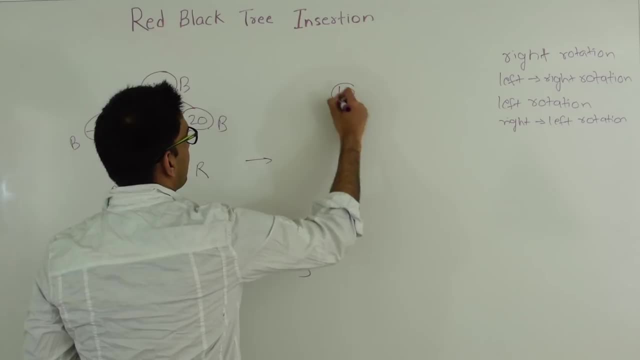 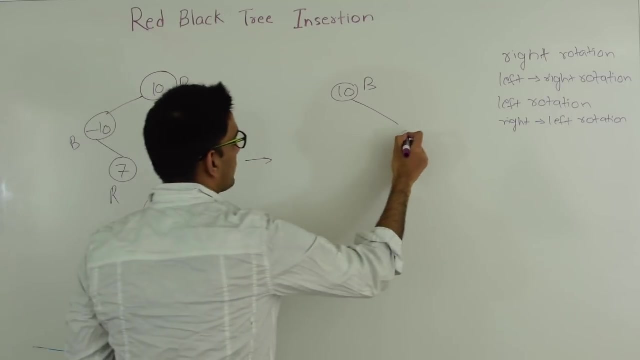 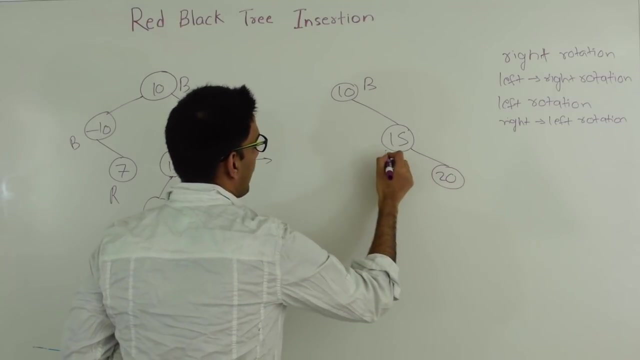 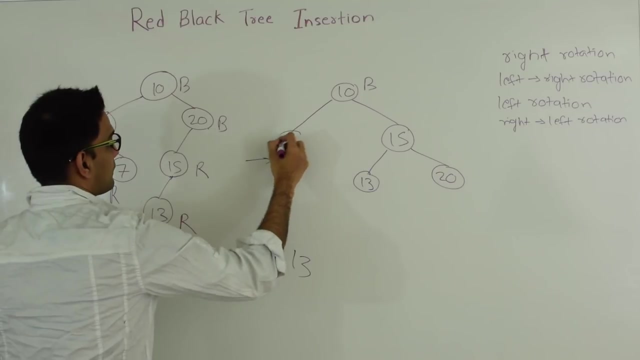 So 10.. This is black. Now, 10's right child will be 15, because we are doing a rotation at this point. Its 15's right child will be 20.. 15's left child will be 13.. And rest of the tree will stay same. 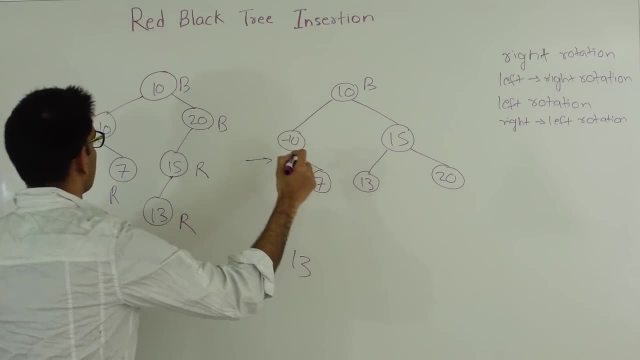 So black-red-red. Now what we are going to do is we are going to switch the color of these two nodes. So this node was red before, Now this will become black. And this node was black before, And now this will become red. 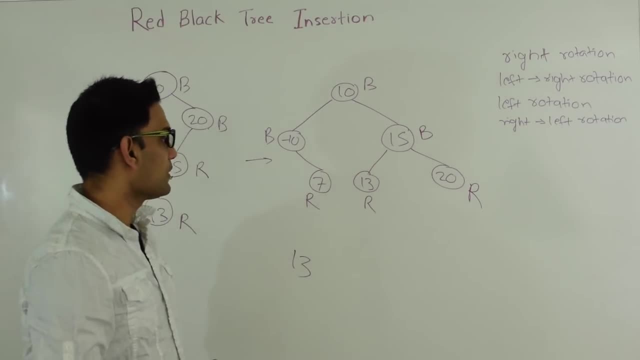 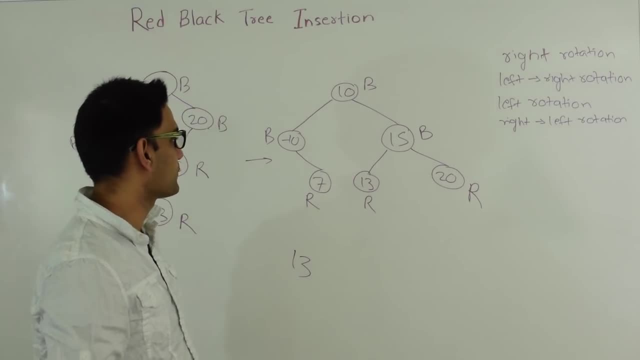 This is 2. And then there is no red-red conflict And the root of this tree is black. So this is a red-black tree. I will later on show why rotation works. Now let's look at a quick example of left rotation, followed by a right rotation. 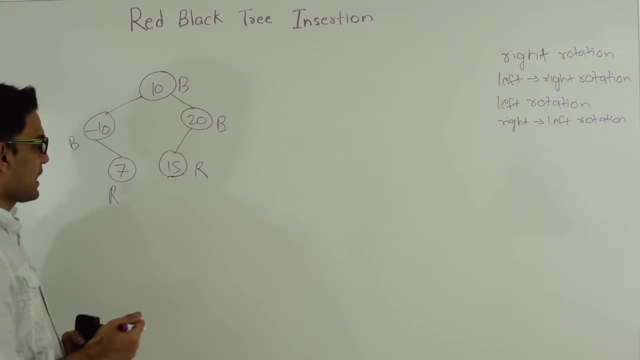 So same tree as before. This time I will try to insert 17.. So 17 is greater than a 10.. 17 is less than 20.. 17 is greater than 15.. So 17 goes right here And it's a red node. 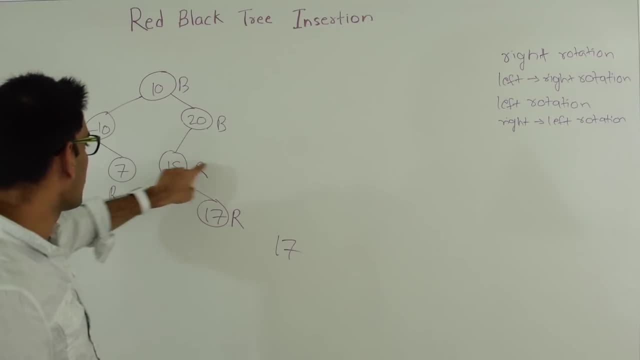 So there is a red-red situation here. We look at its sibling. The sibling is missing, So we have to do rotation. We just need to decide what rotation we need to do. So now, its parent. This is a left child of its parent. 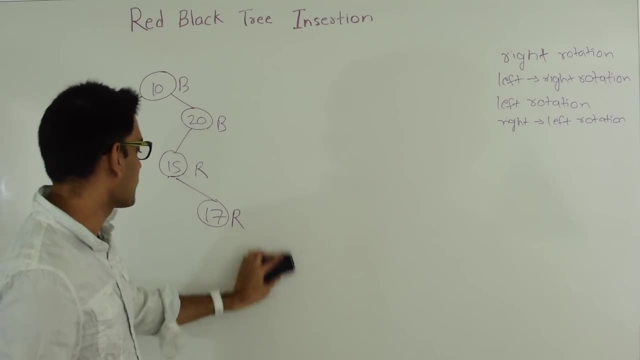 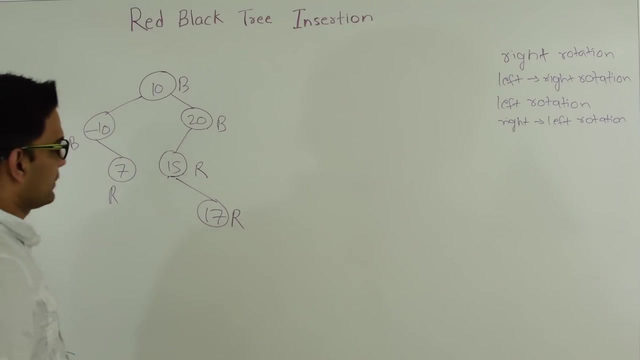 And 15 is left And 17 is a right child of 15.. So in this case, first we have to do a left rotation And then we have to do a right rotation. So the left rotation. here we will do a left rotation at this point. 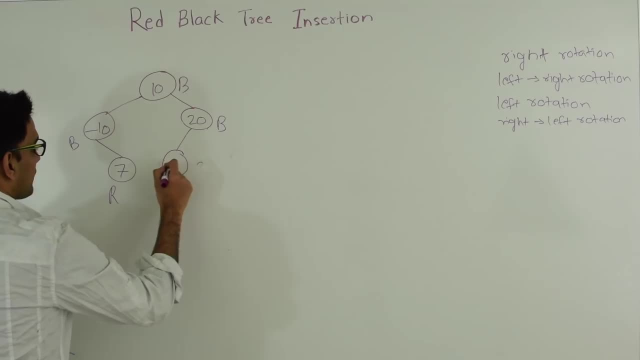 So what that means is this will become 17.. And this will become 15. And their color will still stay the same. So now this becomes A situation like before, And now we are going to do a right rotation, One right rotation. 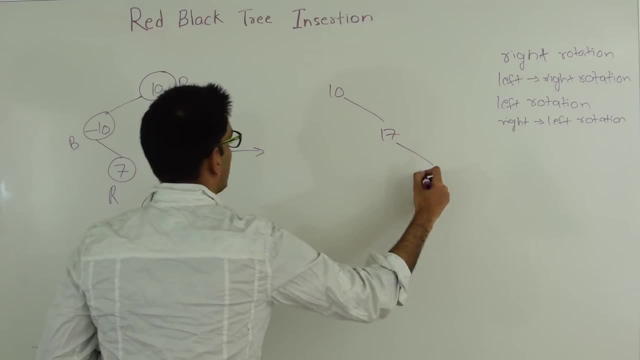 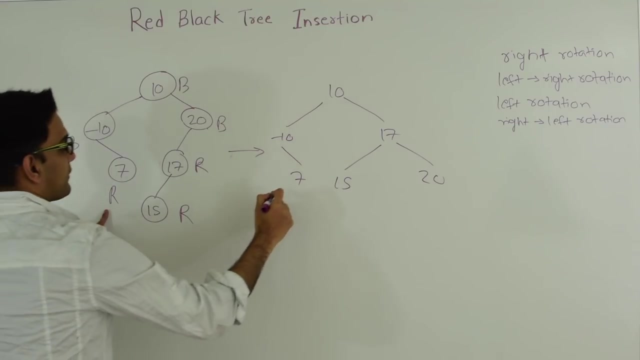 So that means this will become 17.. 20.. 15. Minus 10. And 7.. Color of 7 is red, Color of this is black, Color of this is black. Color of 15 stays red And then, just like before, we are going to flip the color of 17 and 20.. 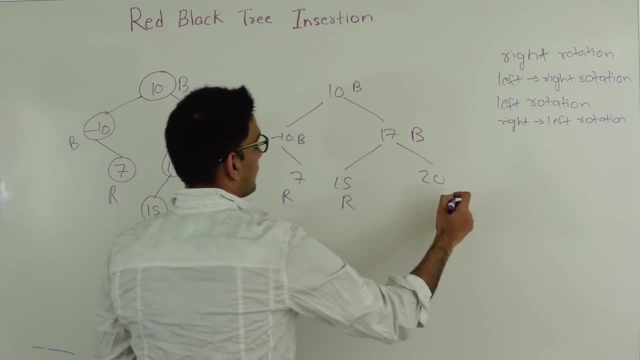 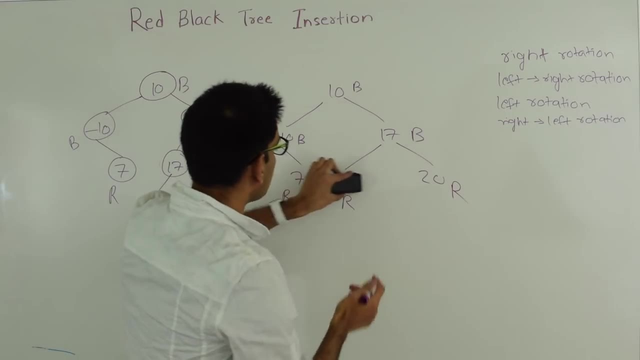 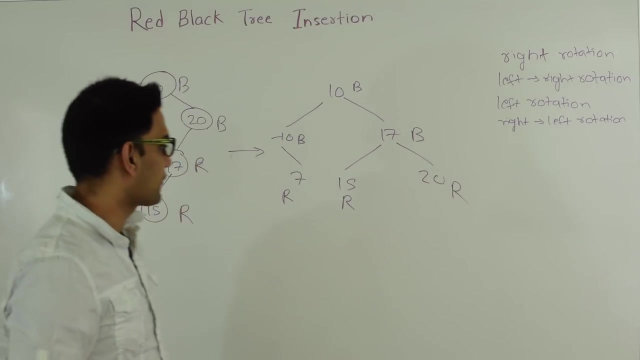 So the color of 20 becomes black, And color of 17 becomes black And color of 20 becomes red. So this is a red black tree now. So the rotationthe left rotation and right rotation, followed by left rotation, are the mirror cases of this. 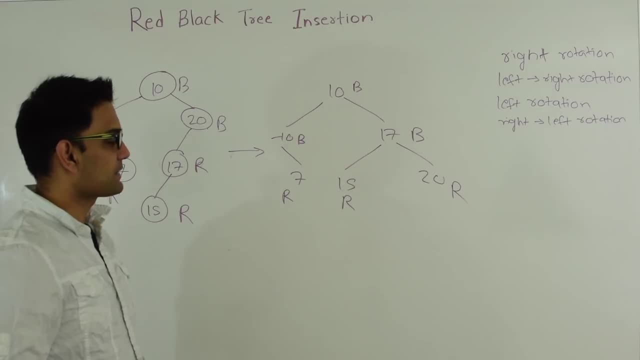 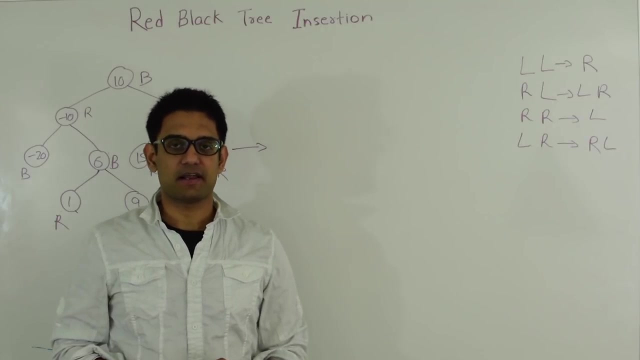 So I am going to skip them in this video. So next let's see what happens if the sibling is black. When a new leaf node is inserted as a red node, its parent's sibling is either going to be missing or it will be red. 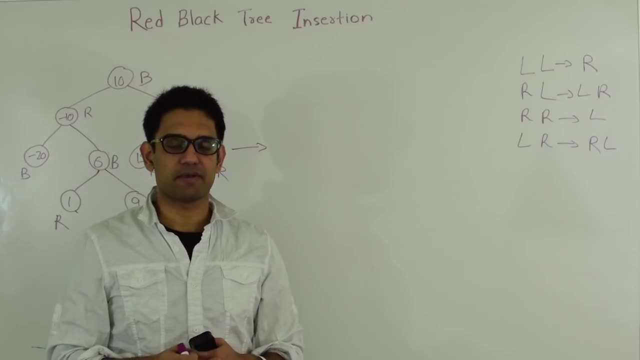 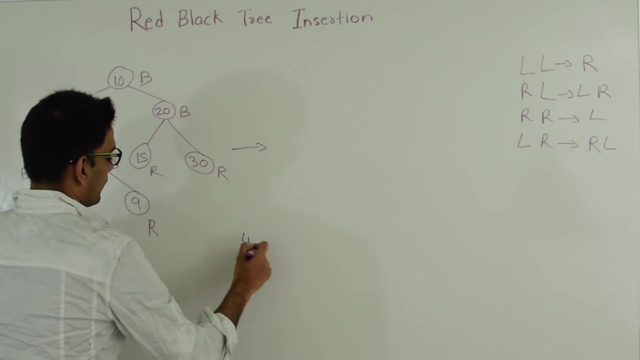 It will never be a black node to start with, But once we do some recoloring then it might end up being a black node. Let's understand with this example here. So here I try to insert 4.. So 4 is less than 10. so we go on the left. 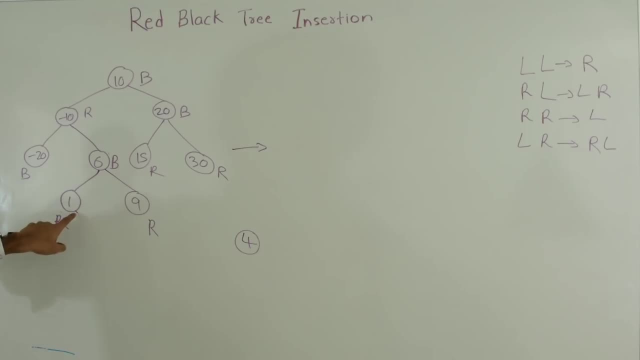 4 is greater than minus 10, so we go on right. 4 is less than 6, so we go on left. 4 is greater than 1, so we go on right And we create 4 as a right child. So this created a right, right situation. 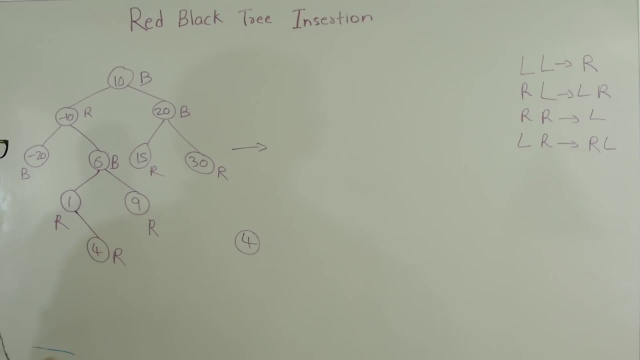 So we look at this guy's sibling. This is also right. So, as we discussed before, we will do a recoloring and make this black and black and this as red. So it fixed the red red situation here, but it created a red red situation here. 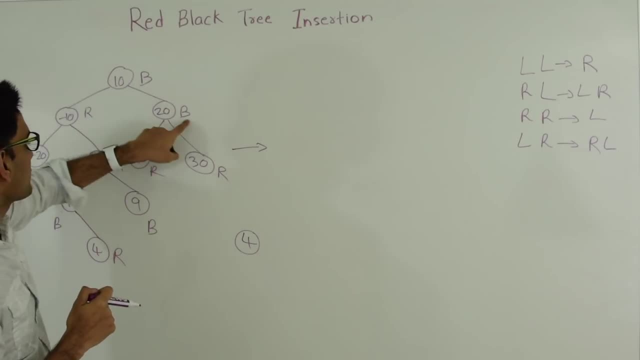 So now again, we are going to look at this: This guy's sibling. So this guy's sibling, in this case, is black. So what we are going to do is we have to do some rotations. So to decide what rotation to do is, we have to look at the positions. 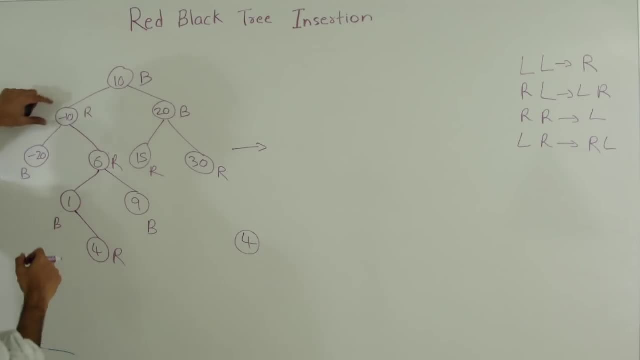 We have to look at what child this minus 10 is. So minus 10 is a left child of 10, while 6- the point at which the conflict is happening- is a right child of minus 10.. So what we are looking for is, since 6 is a right child, 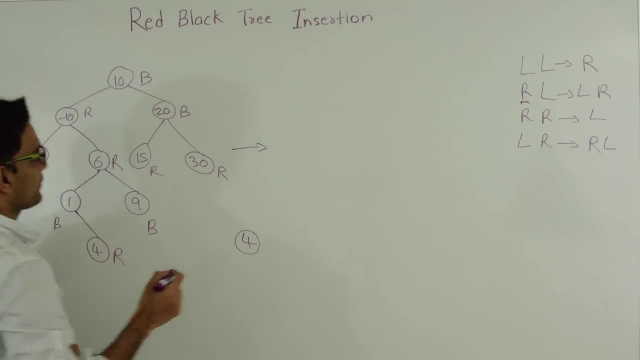 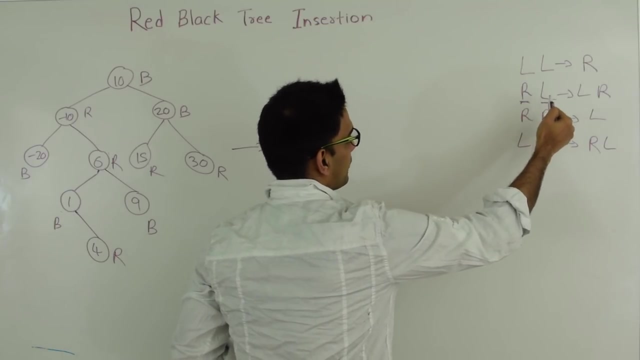 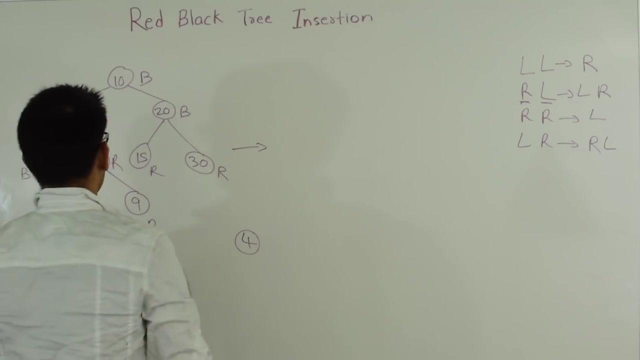 We have this right. and since minus 10 is a left child of 10, we have this left. So when we have a right child and it itself is a left child of its parent, first we have to do left rotation, followed by right rotation. So first we are going to rotate here and we are going to do a left rotation. 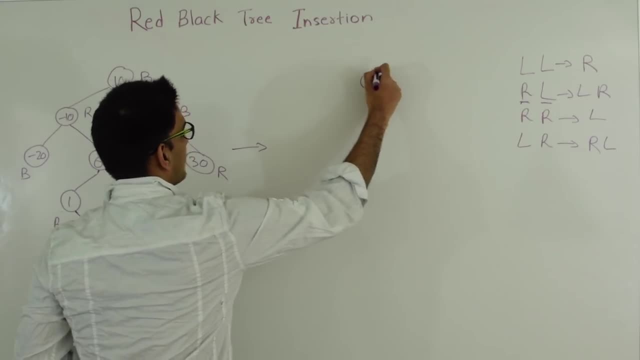 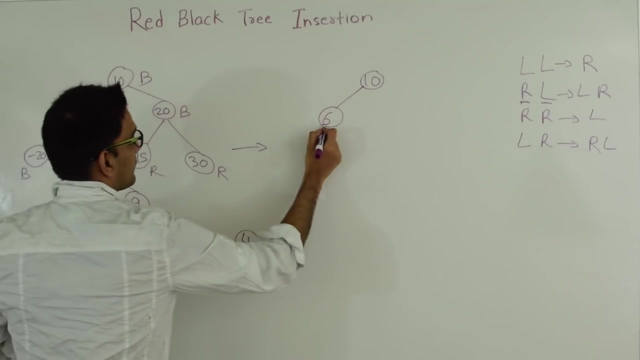 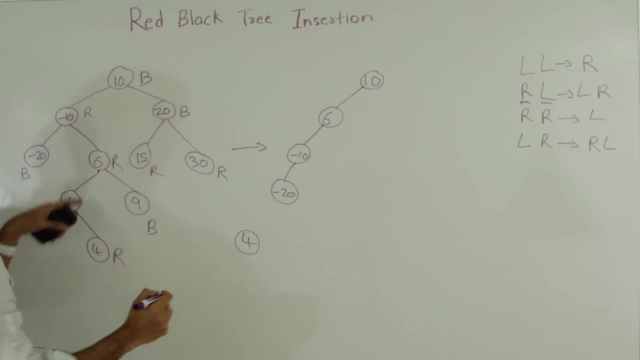 So let's do that. So 10 stays the same as before and we are going to do a rotation here. So 6 comes here, Then minus 10 goes here, Then minus 20 goes there. 1 becomes the right child of minus 10.. 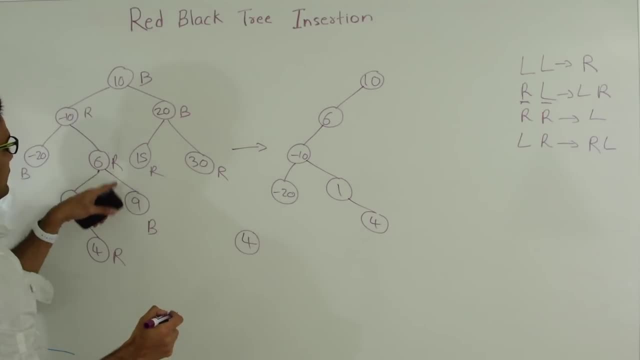 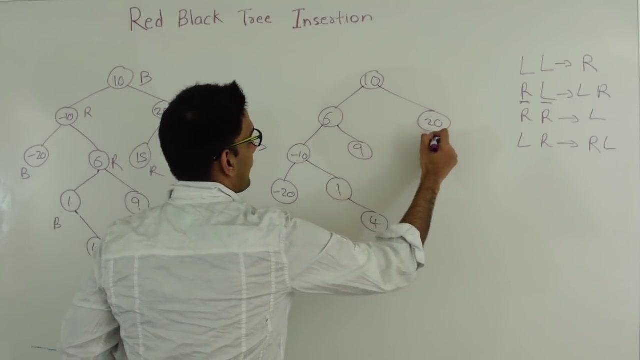 4 stays wherever it is, And then 9 stays with 6. And then its right side stays the same. So when we did thatwhen we did the first left rotation in this, we did not change their colors, So their color stays the same. 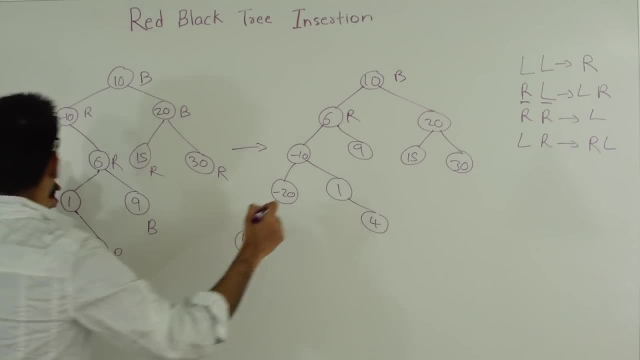 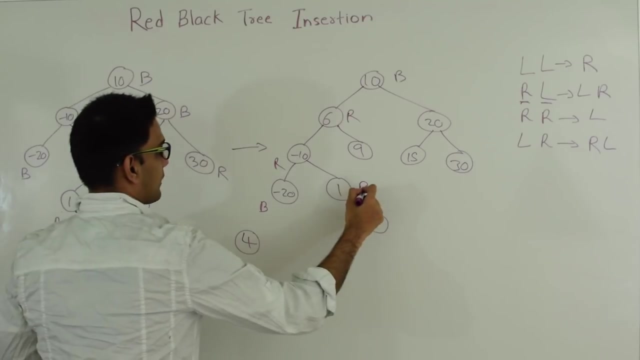 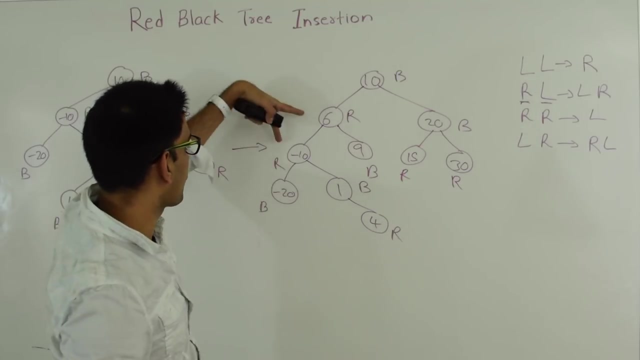 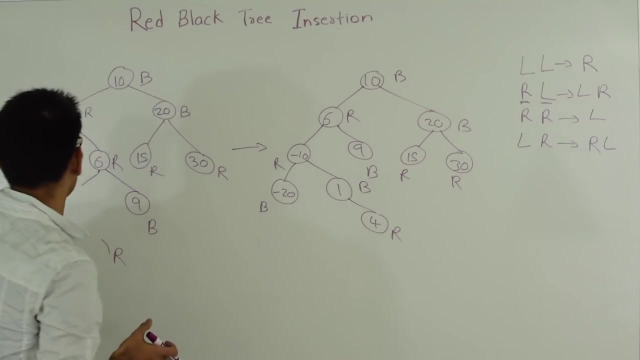 Bredredblack,1 is black,4 is red,9 is black,15 is redred and black. So we still have this redred situation here. So after we did our first left rotation, then we are going to do a right rotation here. 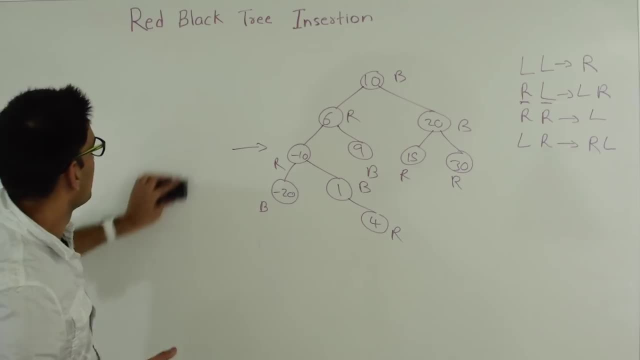 So what that means is we are going to rotate everything on the right. so that means 6 will become the new root, 10 will be its right child. 10's right child will be 20.. 15,30. And 9, which was the left child ofwhich was the right child of 6, will become the left child of 9.. 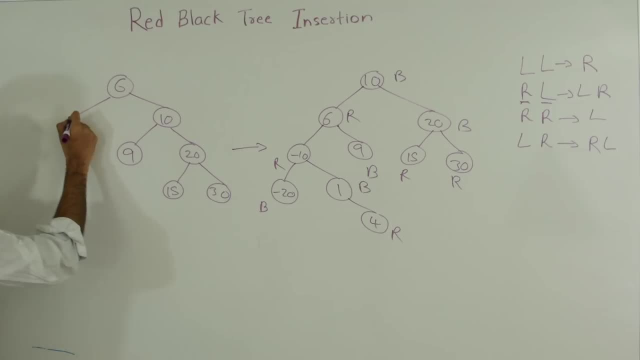 Will become the left child of 10.. And on its left sideminus 10,minus 20,1 and 4.. Let's add their colors, So this will stay red. This will stay black. 9 is black, 20 is black. 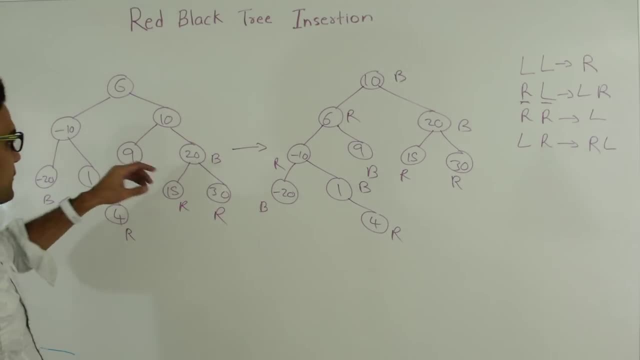 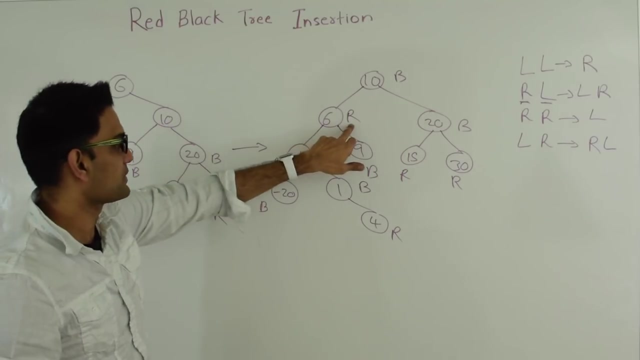 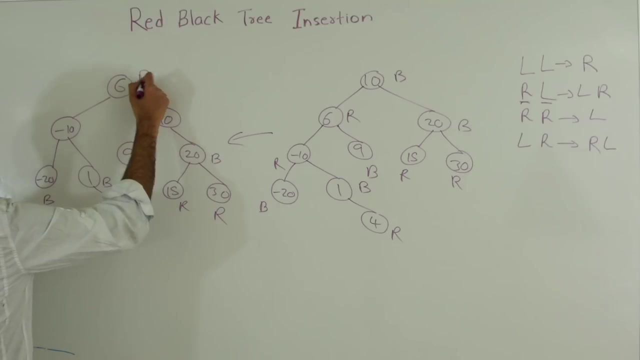 Red and red. So, as we discussed beforeonly thing we are going to do is flip the colors of these two guys. So before rotation this was red, and so before rotation this was red. So this will now become black And this one which was black will now become red. 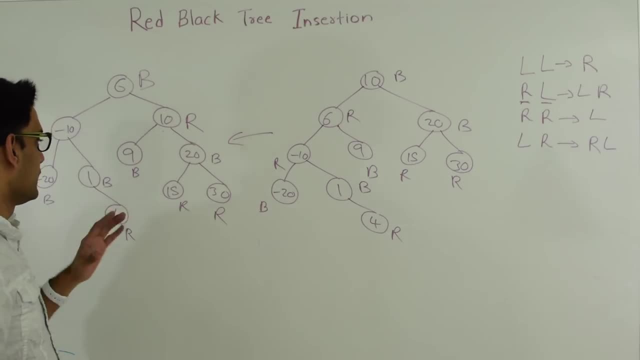 So once we have done this, We are done with the rotation. This again becomes a red-black tree. So let's verify that. So the root is black. There is no red-red relationship. The color of this is red. There is no red-red relationship. 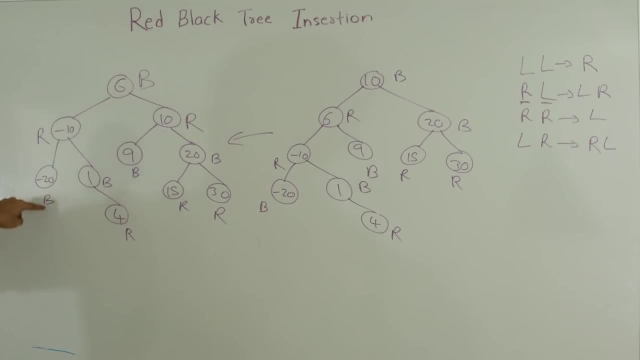 And let's count the number of black nodes on every path: 2,2,2,2,2 and 2.. So this here is a red-black tree. So, as you can see, we had to do a left rotation followed by a right rotation. 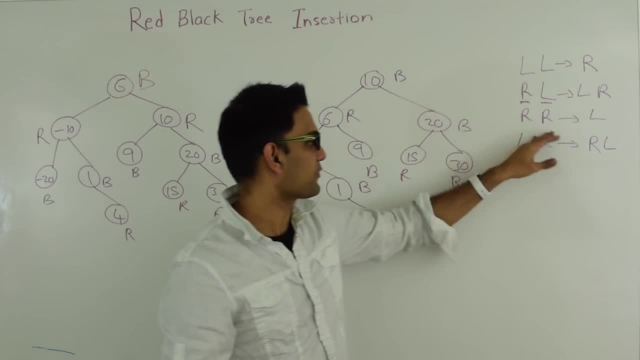 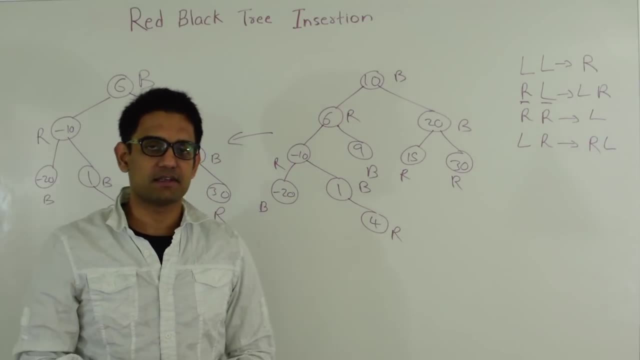 Similarly, if we have a left-left case, we do a right rotation, If we have a right-right case, we do a left rotation, And if we have a left-right case, we do a right-left rotation. So in the next section let's see why this rotation helps in keeping the red-black tree as red-black tree. 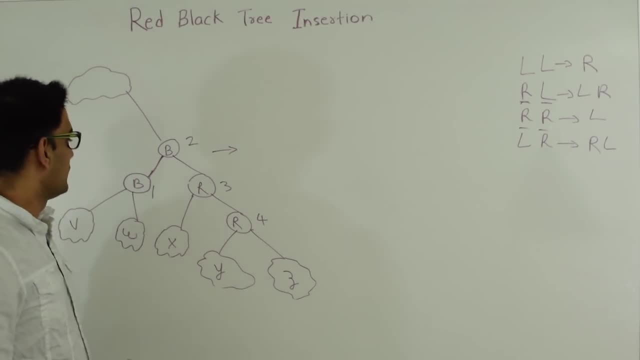 To understand why rotation works, let's look at an example here. So let's assume it's a big tree. All I care about are these four nodes, And they have subtrees under them, And then there is more tree above this level. So now we also note that the number of black nodes from root to every path is same. 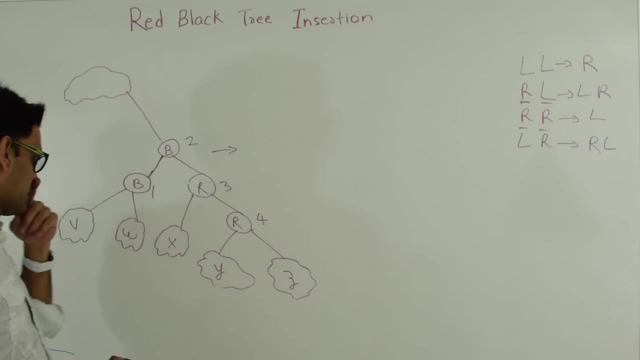 But we have this red-red situation. So in the red-red situation we check its sibling. So this sibling is black. It means that we have to do some rotation. What rotation to do depends on the relationship between them. So this is a right child on the left. 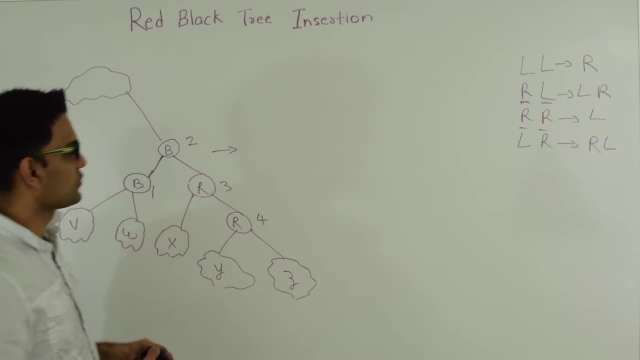 4 is a right child of 3.. And 3 is a right child of 2.. So we have this right-right situation. So we are going to do one left rotation. So now let's assume that total number of black nodes from this point onwards and down is n. 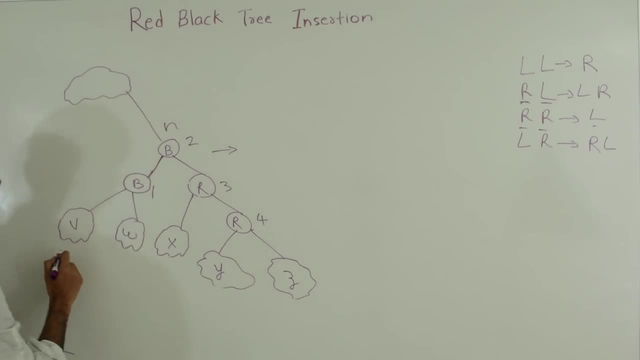 So in this subtree the total number of black nodes must be n-2.. In this subtree it must be n-2.. In here it must be n-1,n-1 and n-1.. Here we have two black nodes here. So in this subtree it must be n-2.. 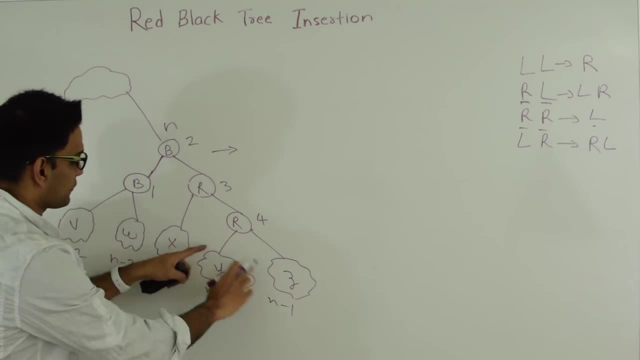 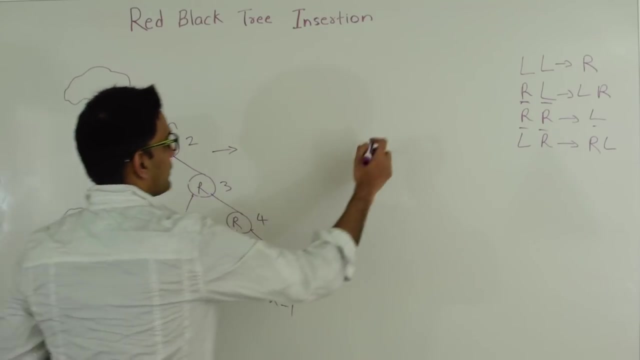 Same here, And here there is just one black node, So it must be n-1,n-1 and n-1.. So now we are going to do a left rotation. So when we do a left rotation,3 becomes the new root. 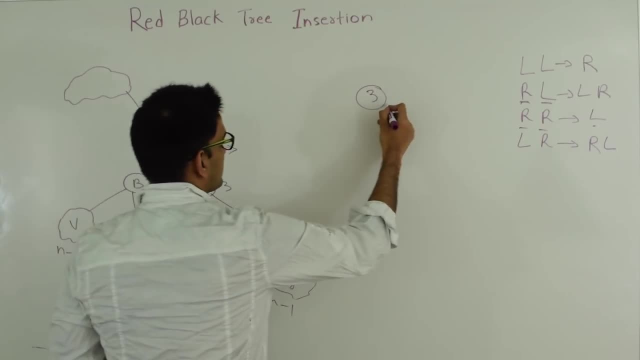 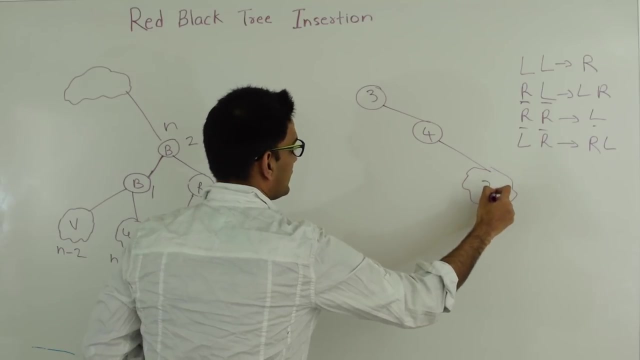 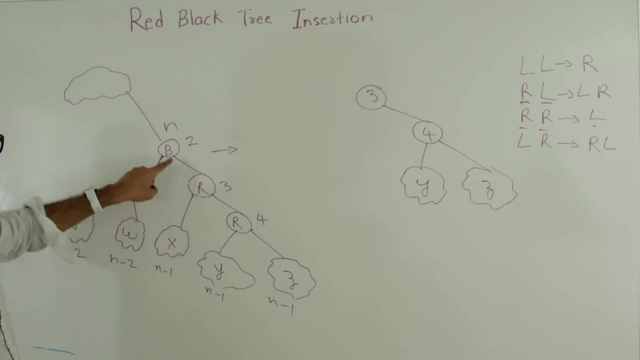 And then its child is 4.. And 4's left and right continue to be same, So z and y. And then this 2 becomes the left child of 3.. And then x, which was the left child of 3, will now become the right child of 2.. 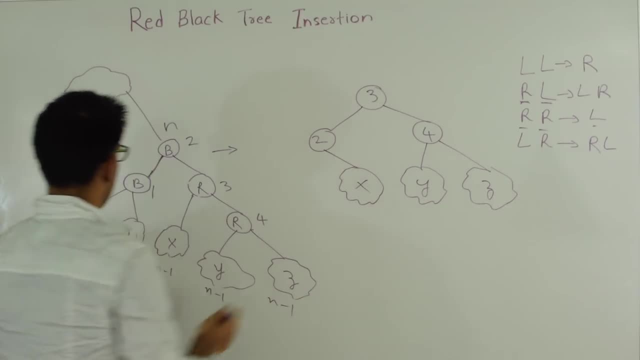 And 1, which was the left child of 1, which was the left child of 2.. Continues to be the left child, And underneath we have v and w. So and then let's do some coloring. So 1 continues to be black. 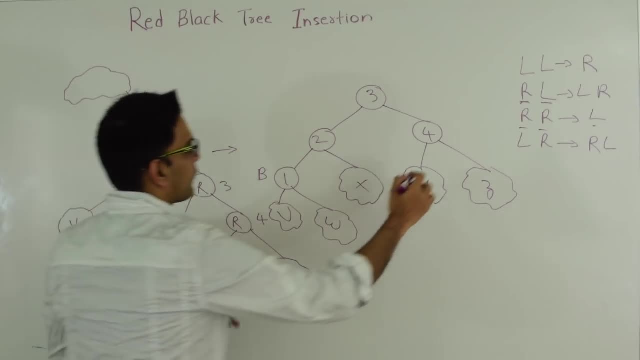 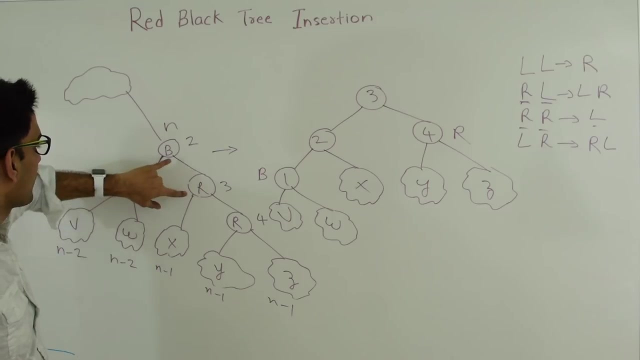 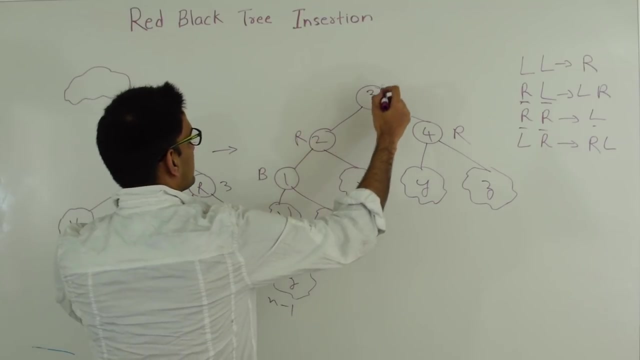 2 and 3. we are going to flip. 4 continues to be red And then, as we discussed before, we are going to flip the coloring of these two guys when we do rotation. So this now becomes.2 now becomes red And this now becomes black. 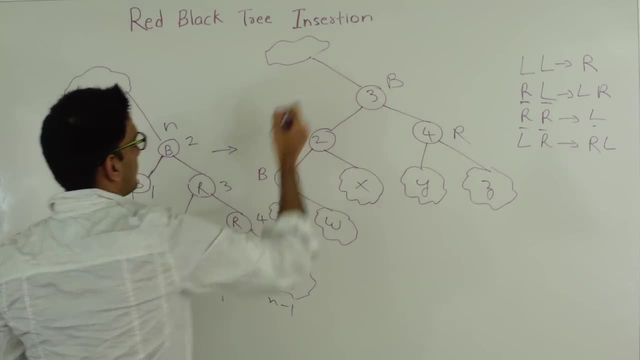 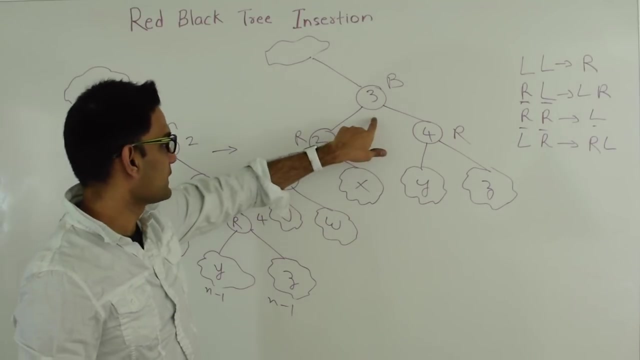 And then there is rest of the tree. So now let's see why this works. So, first of all, since the new root is black, it means that it will never create a red-red relationship with its parent, So we will never have to propagate it. 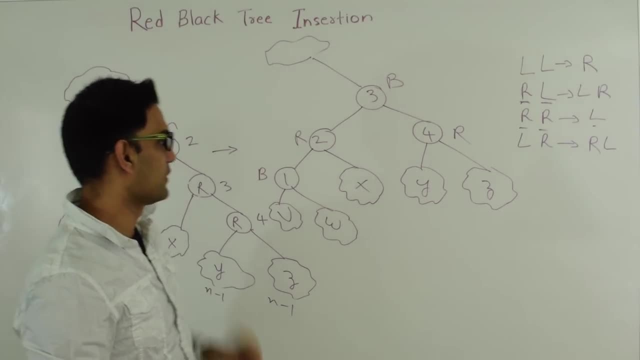 we will never have to check further up, So that is good. So now what we have to check is if are we keeping the same number of nodes or not. So, as we discussed before, the total number of black nodes from here in every path should be n. 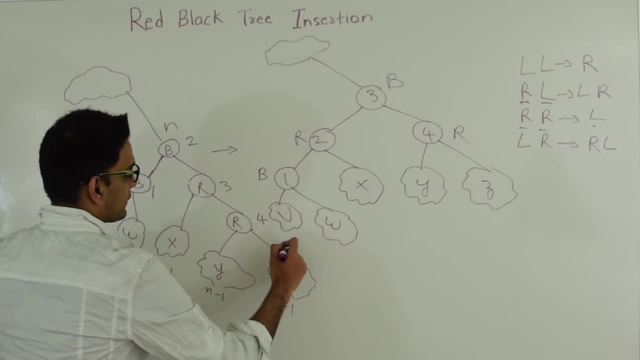 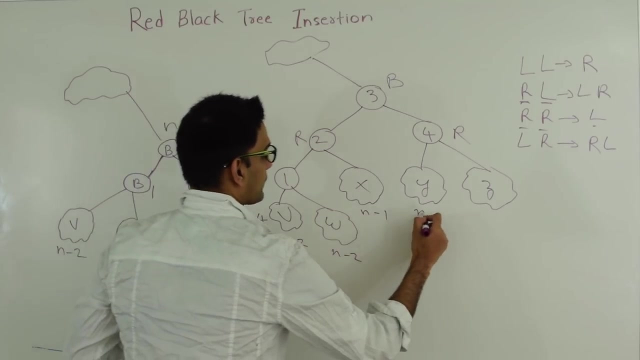 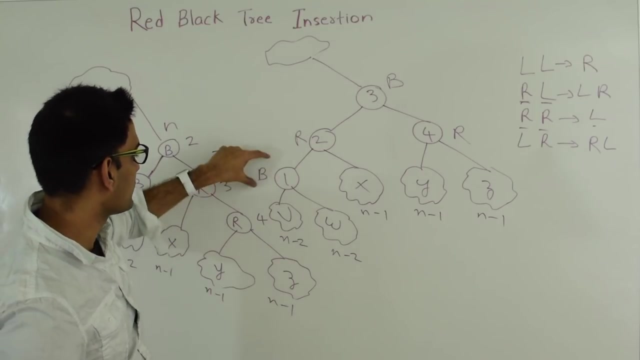 So let's see what happens after this. So in this subtree the total number of left nodes is n-2.. In this subtree it's n-2.. In this subtree it's n-1.. n-1 and n-1.. So now in this subtree here, this is n-2, and then one black node here and one black node here. 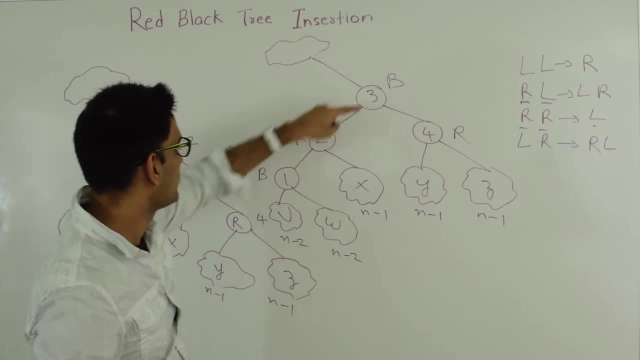 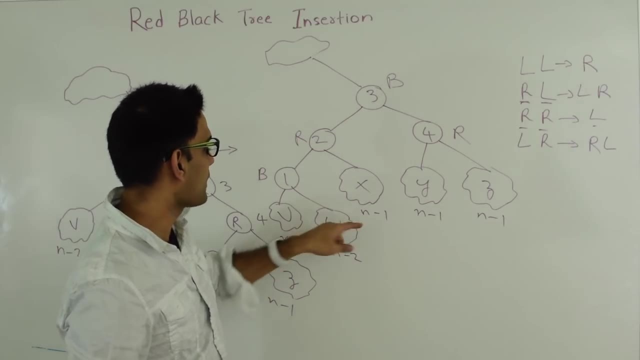 So in this path there are still n black nodes. In this path also, there are still n black nodes In this path. we have n-1 here and one black node here. So still we have n black nodes in this path and in this path. 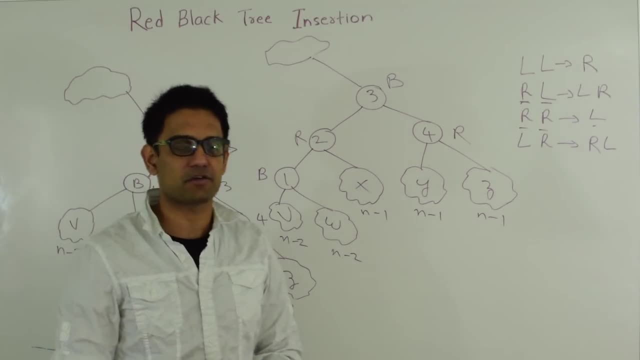 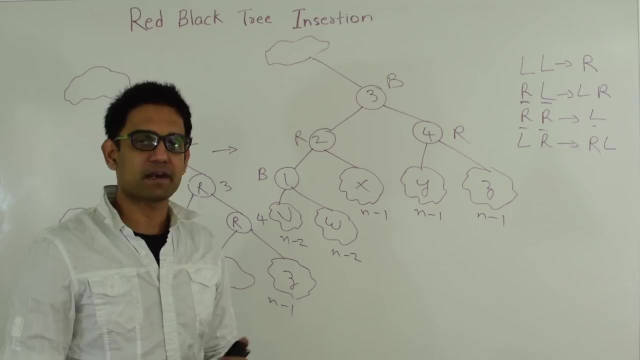 All the path so continues to have n black nodes. So by doing this rotation we continue to maintain the property of red-black tree, that total number of black nodes is same in every path and we don't create any red-red relationship. Also why the red-black tree is more efficient than AVL tree is 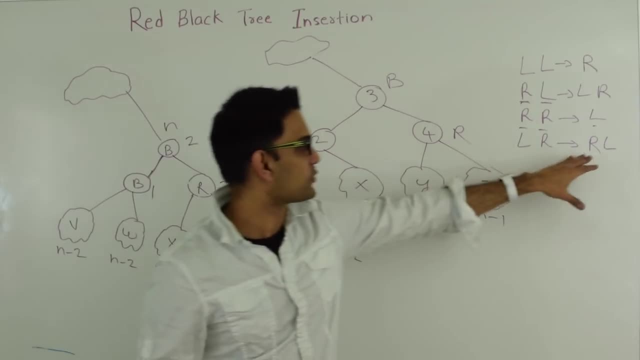 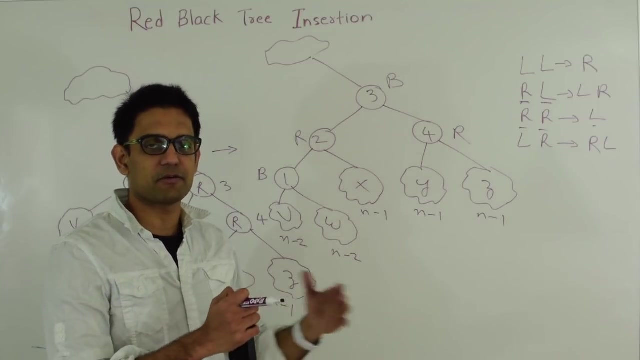 because in red-black tree we just do one or maximum two rotations and then we are done, While in AVL tree we do rotations, we do multiple rotations, and then we might have to recursively fix, we might have to recursively do rotations at the higher level as well. 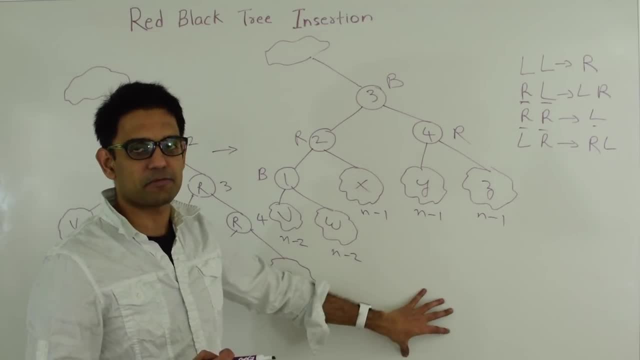 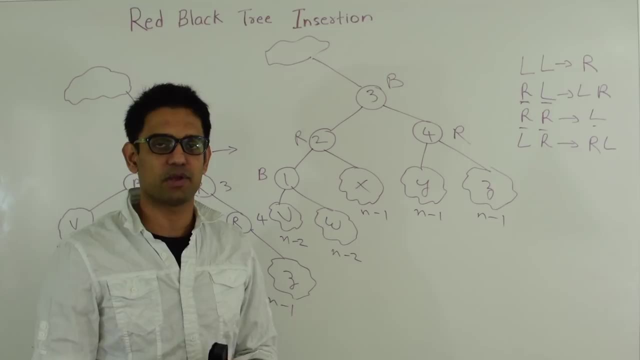 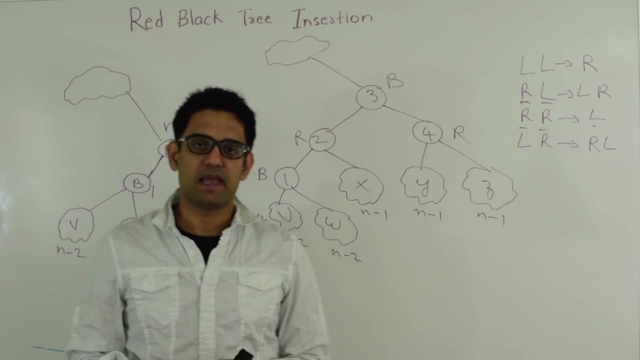 So, which is why in red-black tree is more efficient than AVL tree, because at worst case, in every insert we just need to do, worst case, two rotations, while in AVL tree we might end up doing lot more rotations. So, finally, let's look at one example and then wrap it up with looking at the code of red-black tree. 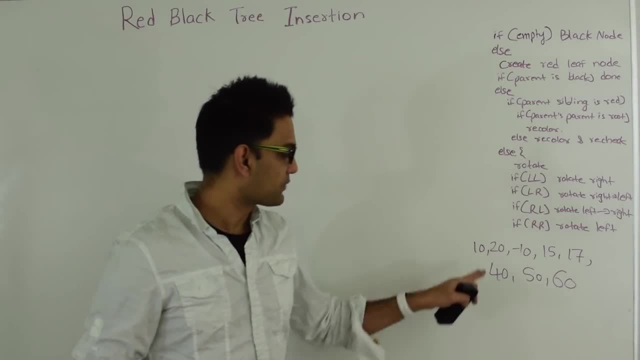 Let's do one final example by creating a red-black tree from scratch using these elements. This is the algorithm of red-black tree in very concise form. So let's start with 10.. Tree is empty at this point of time, so we are going to create one black node. 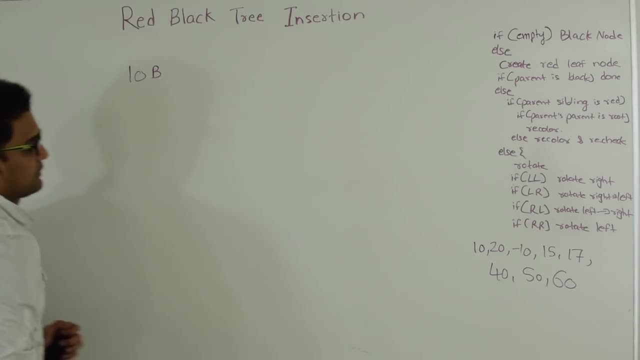 So 10 and this is black. Now we try to insert 20.. 20 is greater than 10, so a new node is always created as a red node And then we are going to check. if parent of this newly created node is black, then we are done. 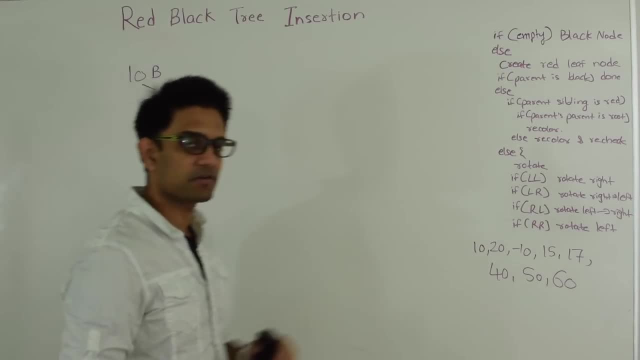 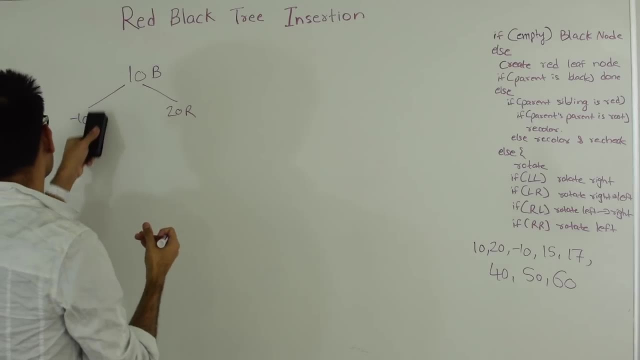 The parent of 20 is black, so we are done. Then we try to insert minus 10, which is less than 10, so it goes as the, it goes as the left child of 10 and its color is red. And then the parent of the newly created node is black. it is. 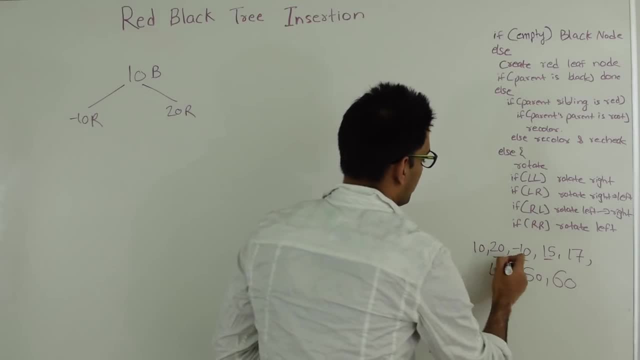 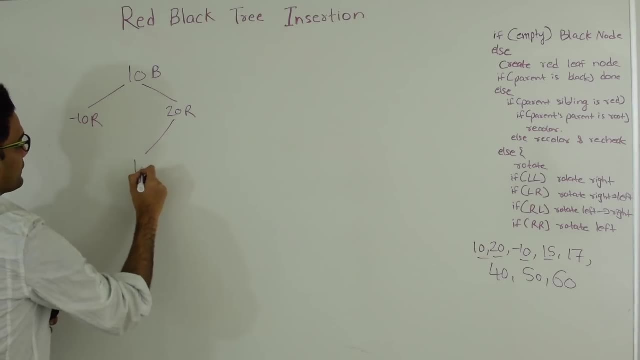 So we are done. Then we try to insert 15.. So 15 is greater than 10,, less than 20.. So it goes as a left child of 20.. Its color is red, So the parent of the newly created node is not of black color. so we go into this else condition. 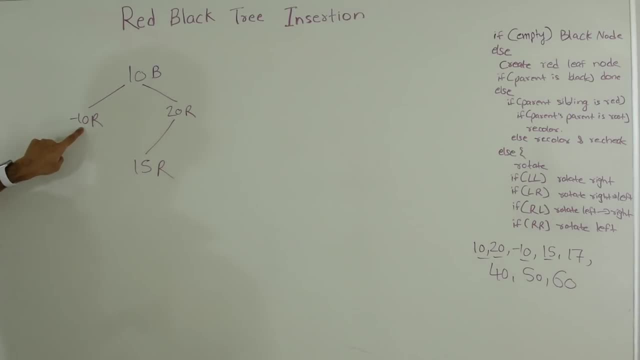 So we check parent sibling. So we look at the sibling of 20, which is 10, and its color is red. So what we are going to do is we are going to do some recoloring So this becomes black, This becomes black. 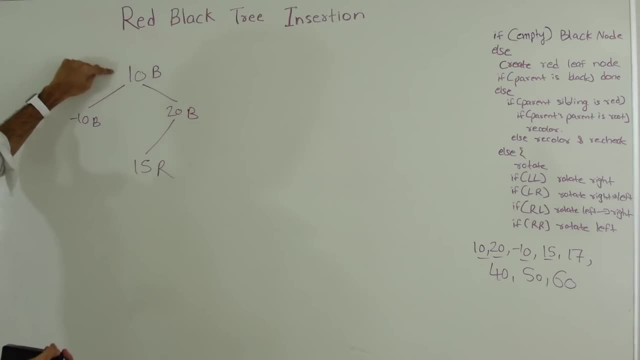 And then, if the root, if 10 was not the root of this binary search tree, we would have changed its color to red, But since it is a root of binary search tree, we will leave its color as black. And now this again is a red, black tree. 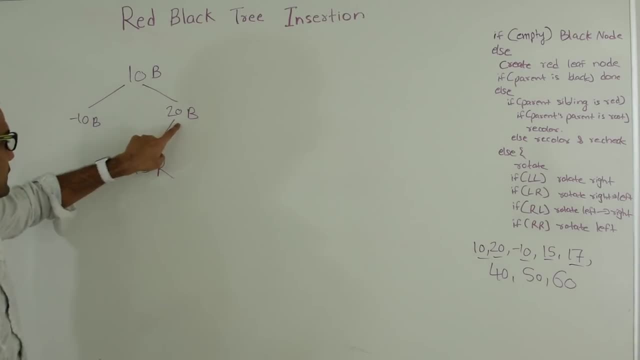 Let's try to insert 17.. 17 is greater than 10, less than 20, greater than 15.. So we come here And its color is red. So now this again created this red red conflict. so we come into this else condition. 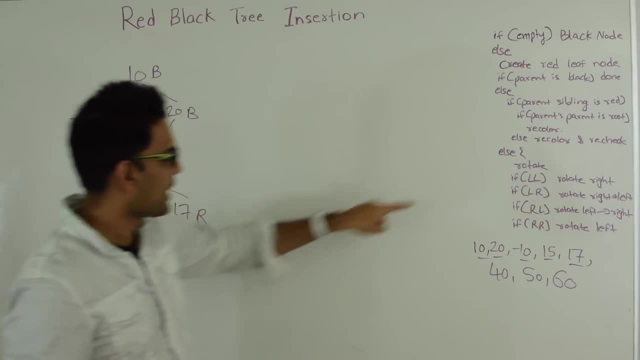 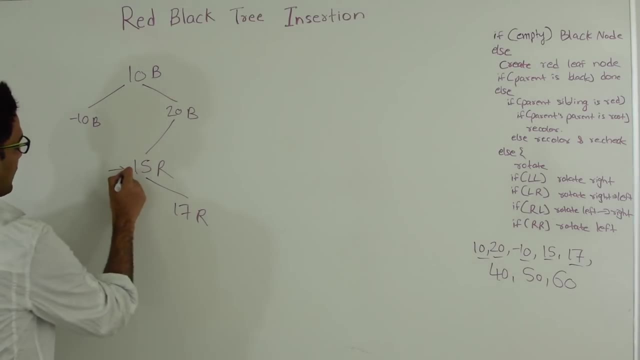 Now this guy doesn't have a sibling here, So we have, we come into this else condition and we have to do one of the rotations. What rotation to do? So we look at this guy, the place where conflict is happening. Its child is a right child. 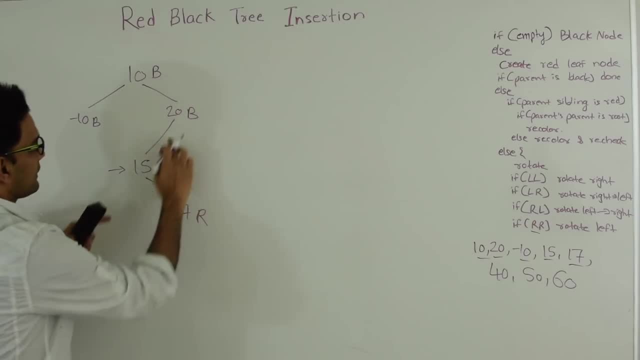 So first is right And it itself is a left child of 20. So second one is left. So right and left. So what we are going to do is we are going to first rotate left, We are going to first rotate left, and then we are going to do a right rotation. 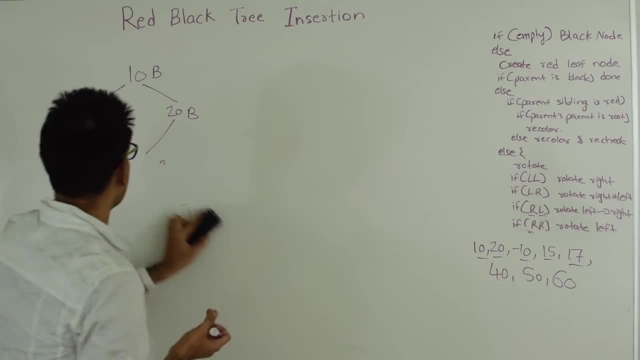 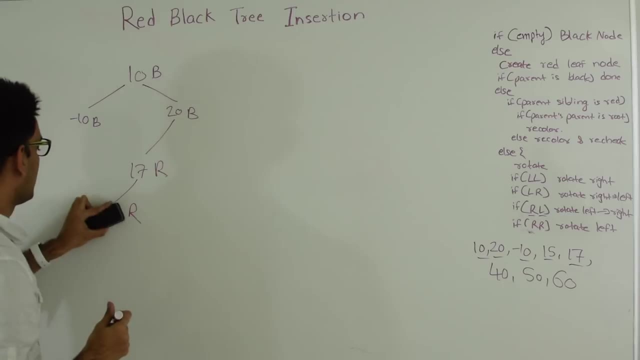 So let's do a rotation at this point. So this becomes So this becomes 17,. red and 15. When we do the first rotation, we are not going to change the color of any node. Now, once we are done with this rotation, we created a left- left situation. 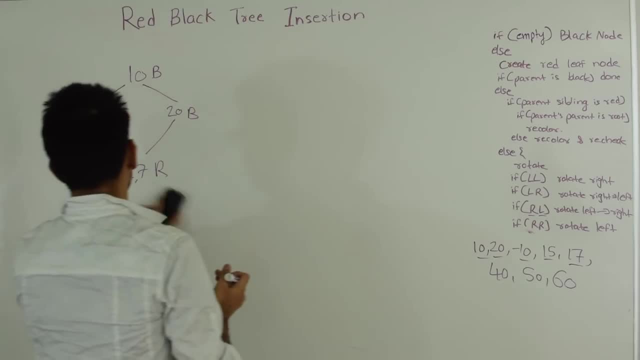 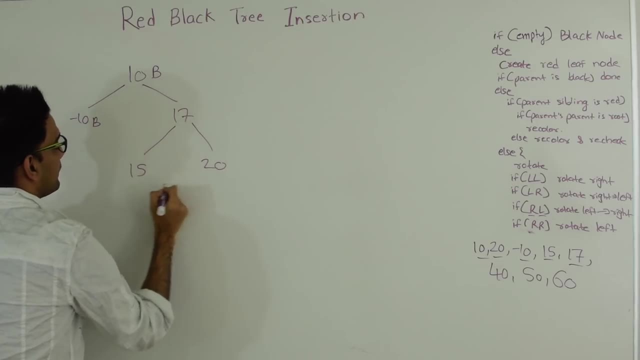 So now we are going to do a rotation at this point, So this becomes 17,, 20,, 15.. And the color of 15 stays the same. Before this rotation, Before this rotation, the color of 17 was red, So we will flip it to become black. 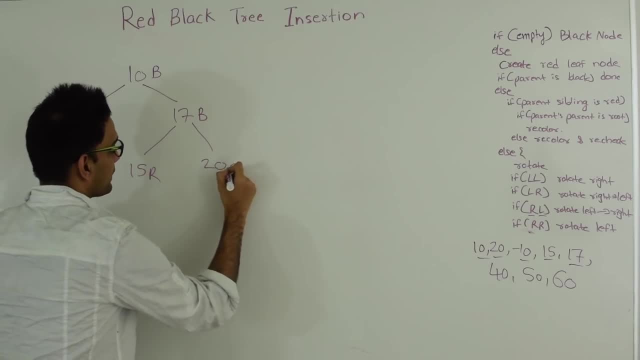 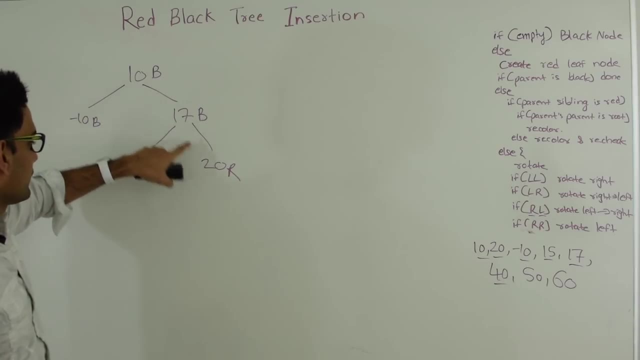 And before this the color of 20 was black, So we will flip it and make it red. So let's insert 40 now. So 40 is greater than 10,, greater than 17,, greater than 20.. So 40.. 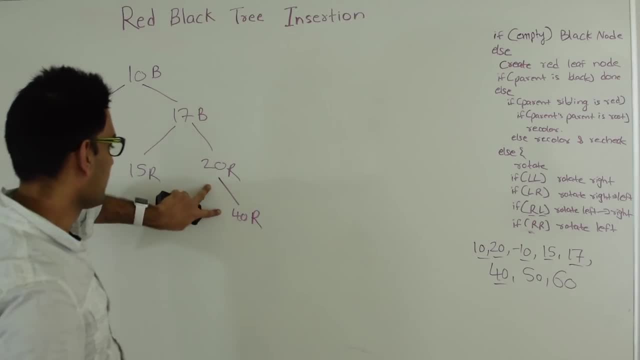 And it's a red leaf. So again, we created this red red condition. So we look at this guy's sibling, which is red. So we are going to do some recoloring here. So this becomes black, This becomes black, And then we go to its parent. 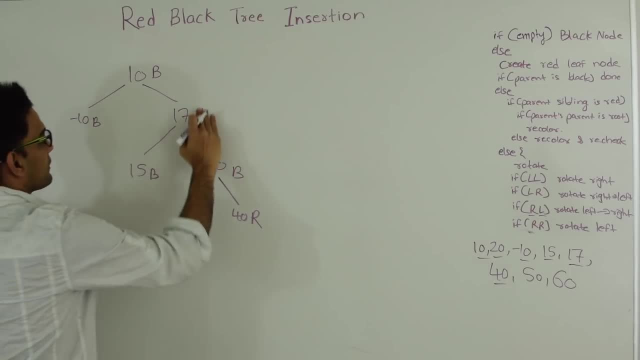 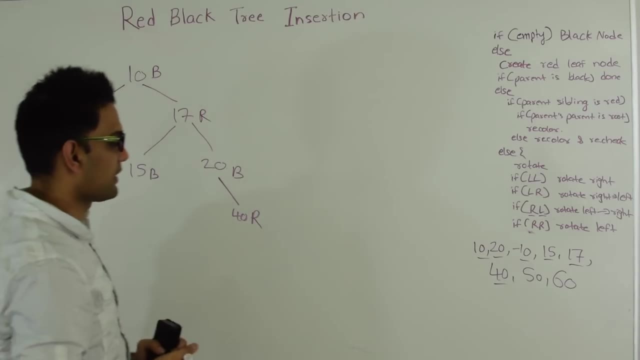 This guy here is not the root of this binary search tree. So we turn this guy's color to red And then we check if we are creating any red red conflict, which we are not, Which means we are done with inserting 40.. Let's try to insert 50.. 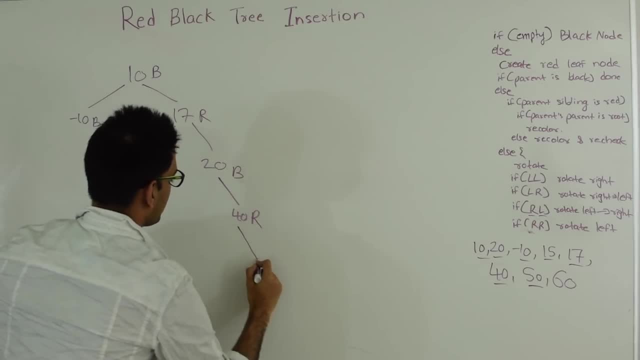 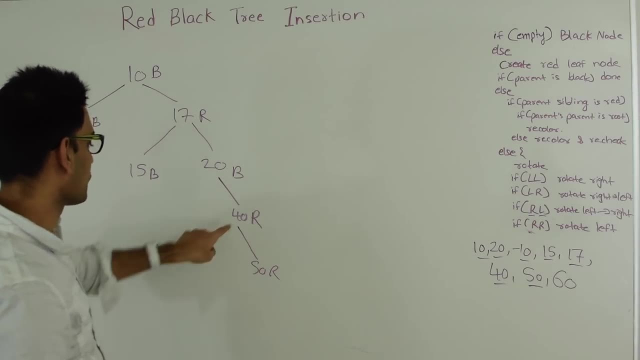 So greater than 10, greater than 17,, greater than 20,, greater than 40 and 50. So we insert it as a right child of 40. So again we created this red red conflict. So we look at 40's sibling which is missing. 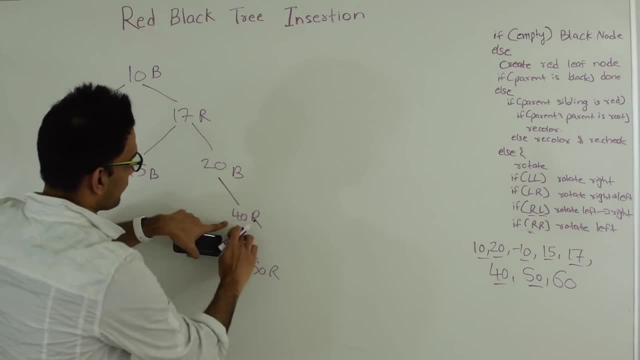 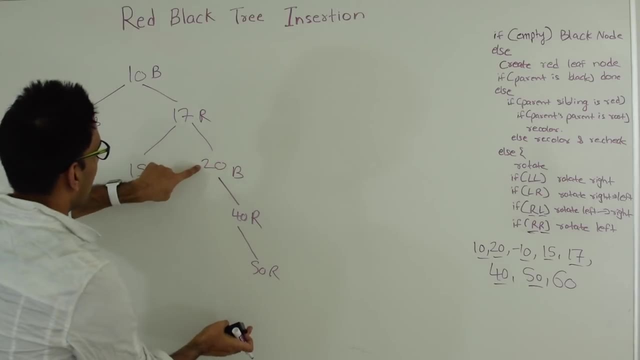 And this is a right white situation: 50 is a right child of 40 and 40 itself is a right child of 20.. So we have this right, right situation. So we have to do one left rotation at this point here. So 40 will become the root here and 50.. 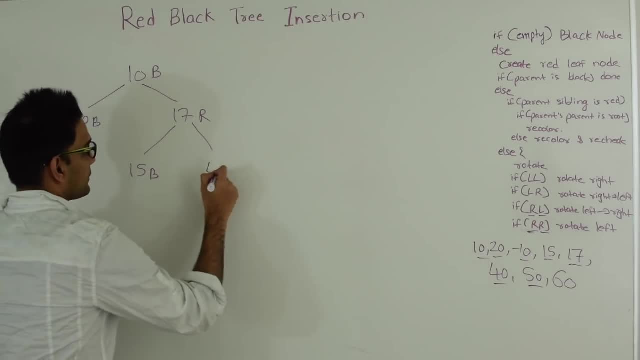 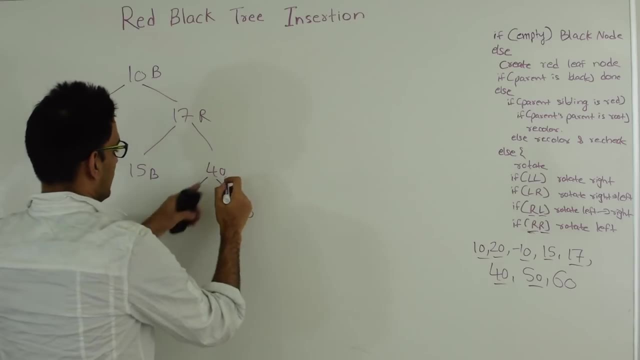 So 40 will become the root here, 50 will be its right child and 20 will be its left child And color of 40 will be And we will flip the color of 20 and 40. So 20 will become red and 40 will become black. 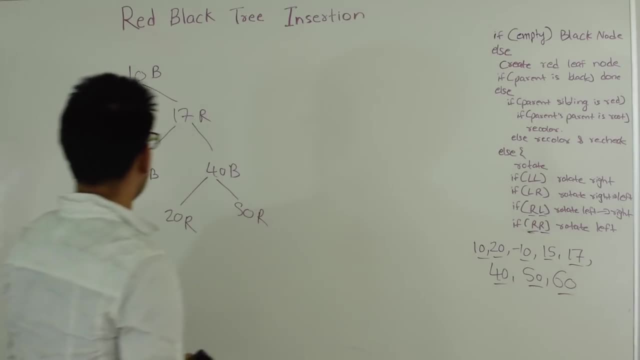 Now, finally, let's insert 60. So greater than 10, greater than 17,, greater than 40,, greater than 50. So we insert it as a right child of 50. This again creates a red, red situation. We look at its sibling, which is also red. 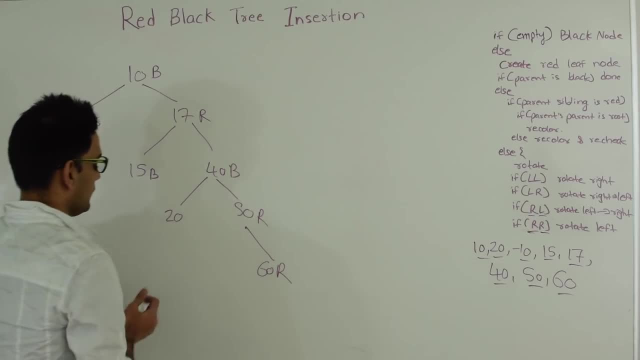 So we are going to do some recoloring, So this becomes black, And this becomes black, And we are going to change this to red because it's not a root of binary search tree. So by doing this, we again created this red, red situation. 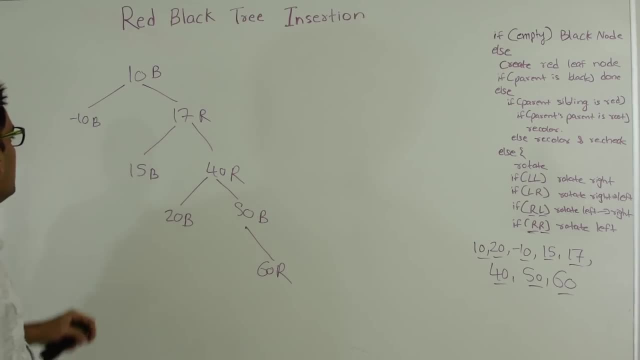 So we are going to look at this guy's sibling, which is black. So now we have to do rotation. So what rotation to do depends on. So 40 is a right child of 17.. So first right. And 17 itself is a right child of 10.. 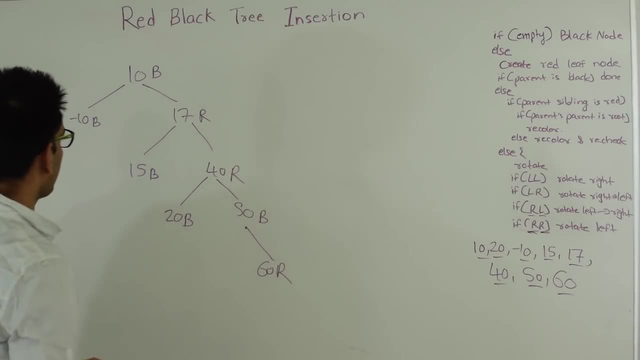 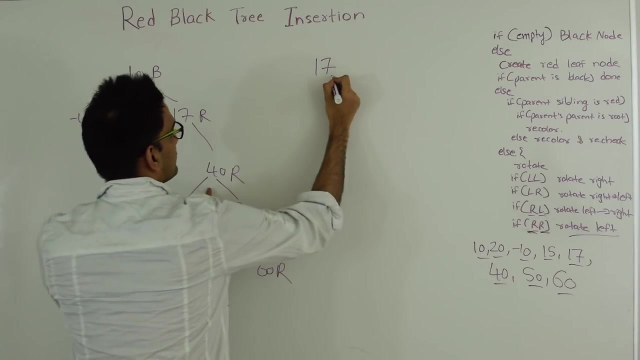 So second right. So what we are going to do is We are going to do a rotation at this point And we are going to do one left rotation. So 17 will become the new root of my binary search tree. Its right side will be 40.. 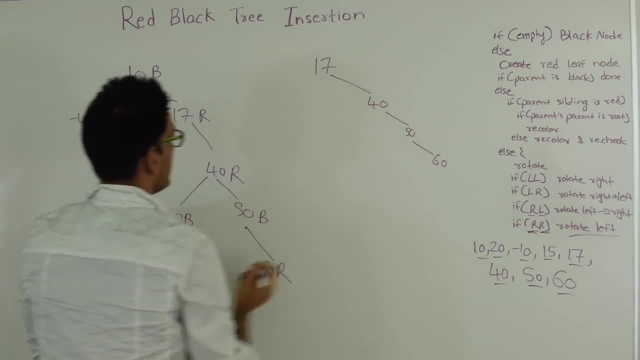 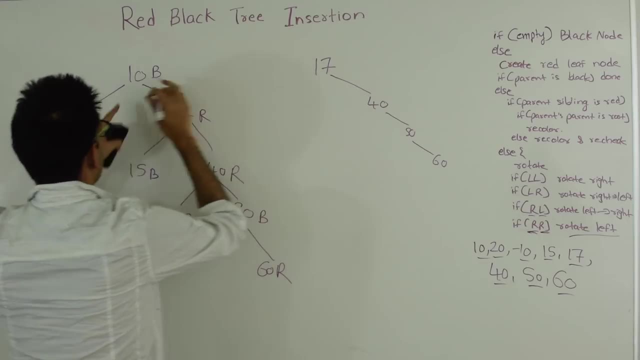 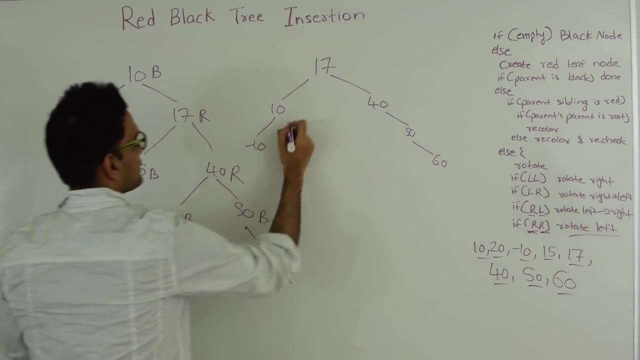 50, 60 Its 15.. 10 will become the left child of 10, will become the left child of 17.. And minus 10 will continue to be its left child And 15, which was the left child of 17 before, will now become the right child of 10.. 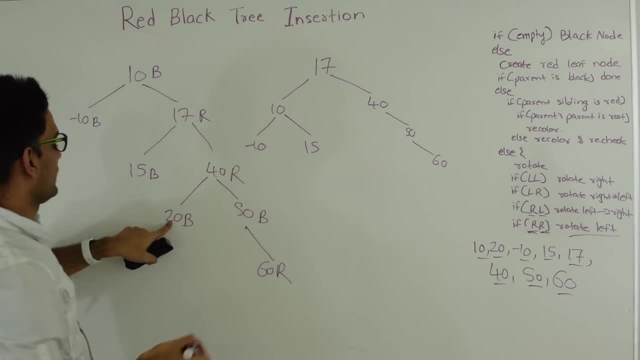 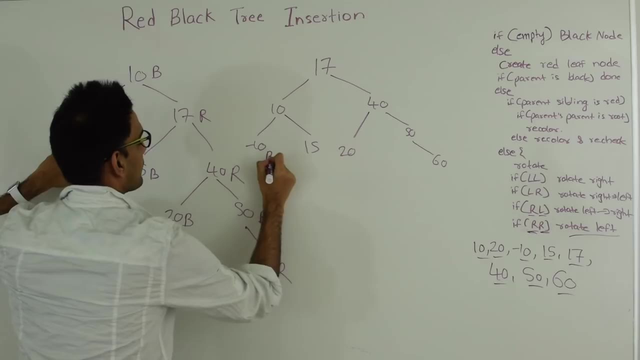 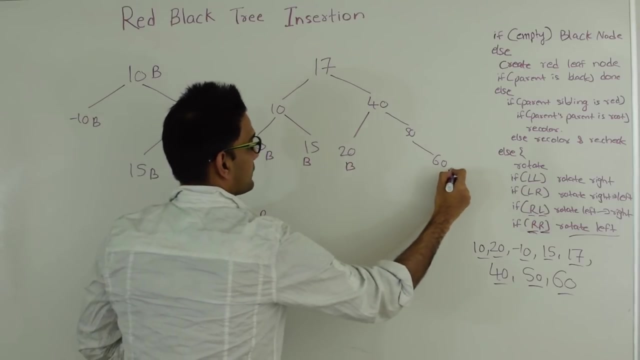 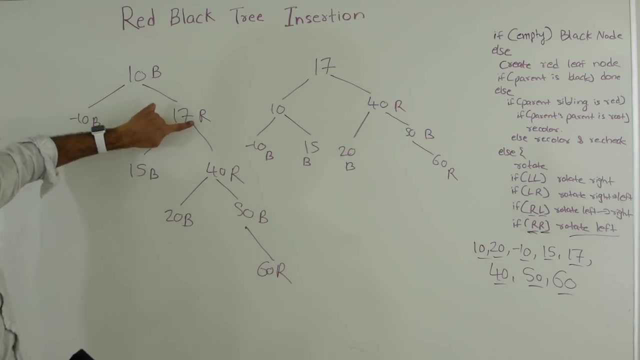 And 20 was the left child of 40. And let's add the color. So this is black, 15 is black, 20 is black, 60 is red, 50 is black, 40 is red. So before rotation the color of this guy was red. 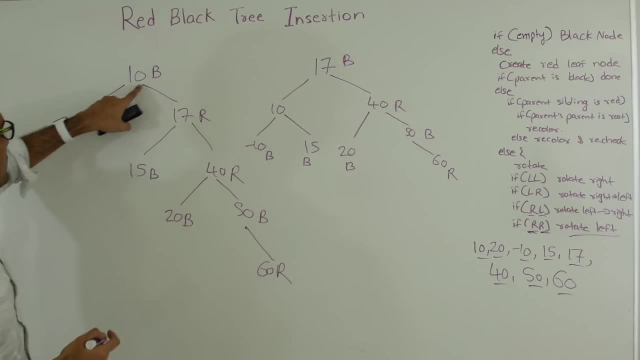 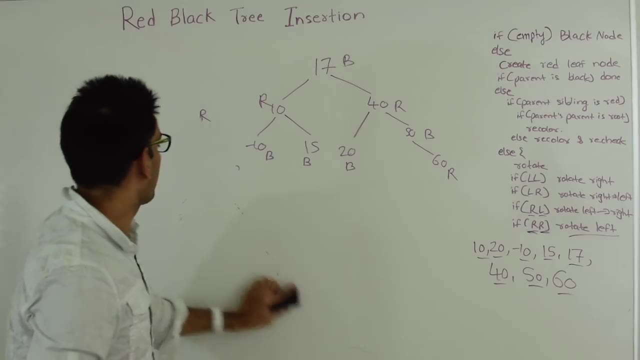 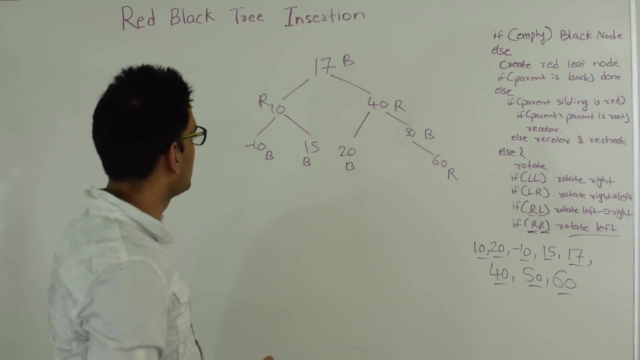 So this will now become black, And color of this guy was black, So this will become red. So this is our final red black tree. Let's make sure that it follows all the properties of red black tree. The root is black. There is no red- red situation. 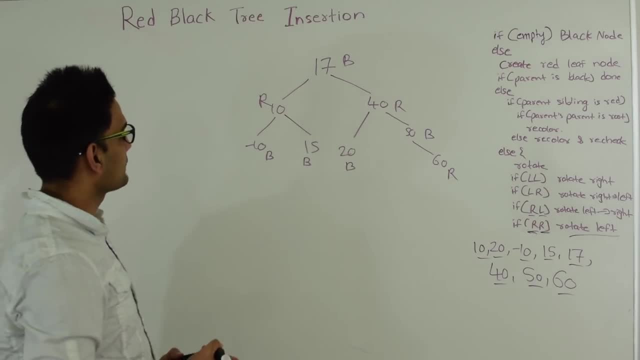 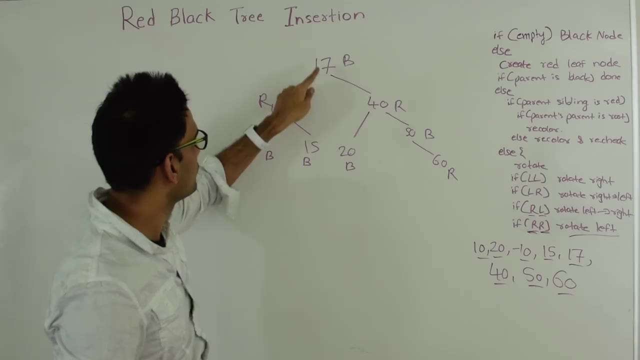 There is no red, red, parent child relationship. And let's count the number of black nodes in every path. In this path, it's 2.. In this path, it is 2.. In here, it is 2.. And let's add a null here. 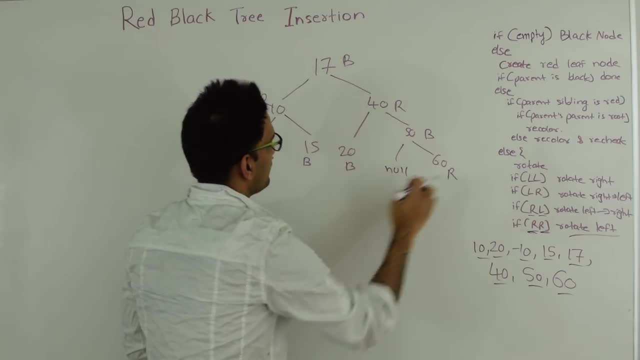 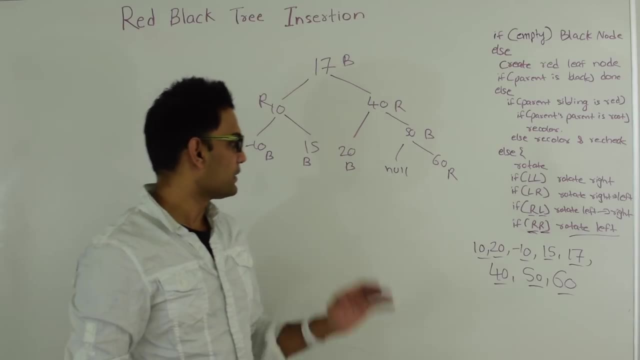 In this path it is 2, and in this path it is also 2.. So it follows all the properties of red black tree. So hopefully, with this example, you understand how we are going to do, how we are doing insertion in red black tree. 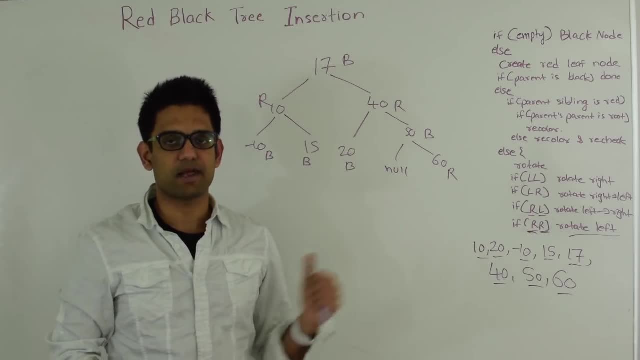 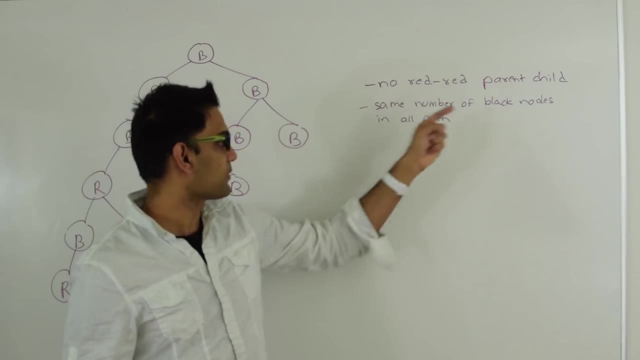 Next, let's try to analyze the time complexity of red black tree. Because of these two properties of red black tree, which is no red, red parent, child relationship and same number of black nodes in all the path, there will never be a path in a red black tree from root to leaf. 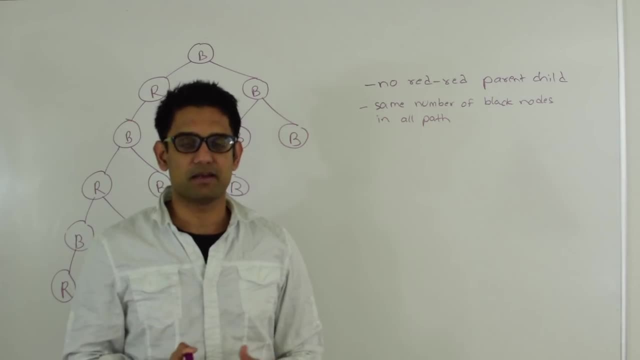 whose length is more than twice of any other path, of any other root to leaf path in red black tree. Let's look at an example here. So this is the worst red black tree. you can have Black node followed by red, followed by black red, black red. 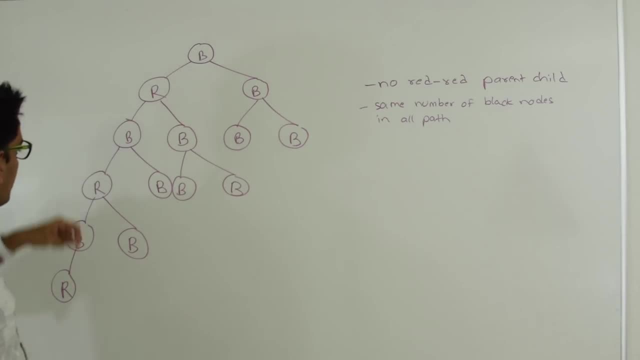 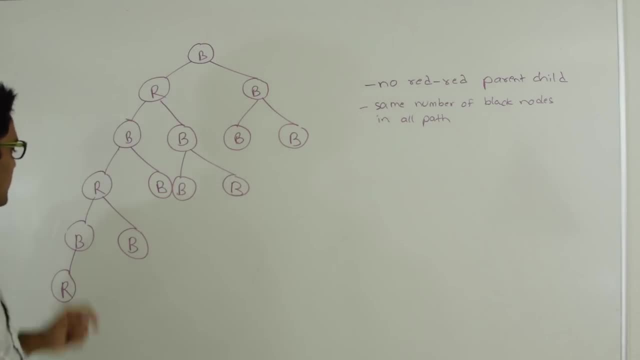 this is 3 nodes: 3 nodes and 3 black nodes. So here you can see, the shortest path here is of length 3, this one or this one, and the longest path is length 6 and because of these two properties, this length here will never be more than twice the shortest length. 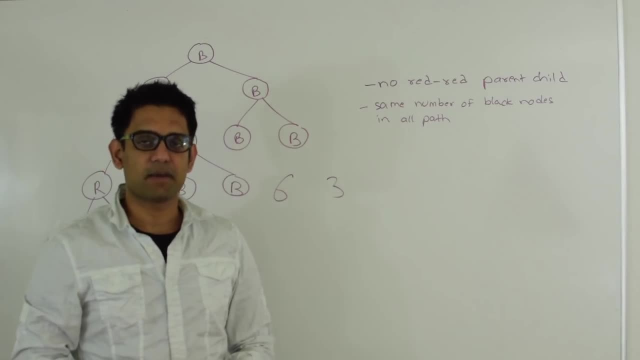 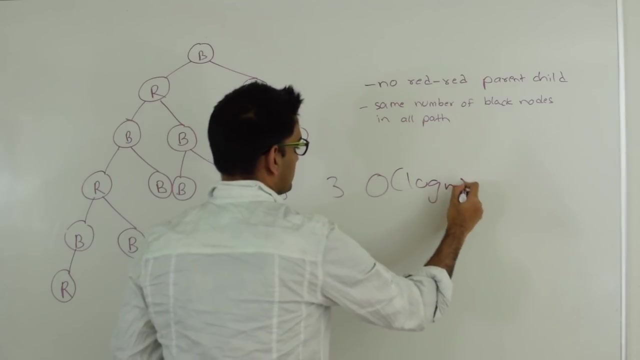 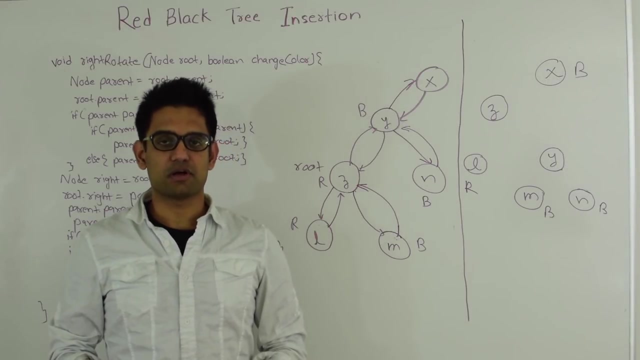 So because of this, the run time complexity for search, insert and delete will always be O of log of n. So next let's look at the code for red black tree. In red black tree, every node, along with having the pointer space to its left and right children, also needs to have a pointer to its parent. 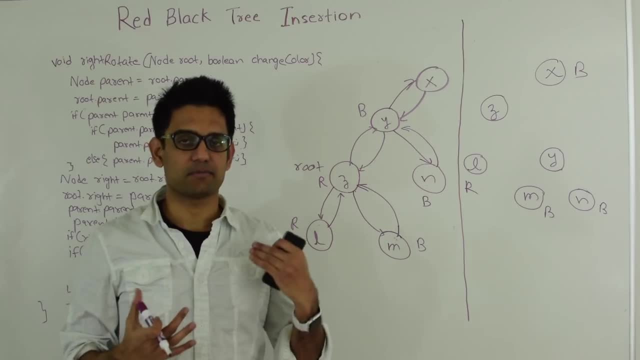 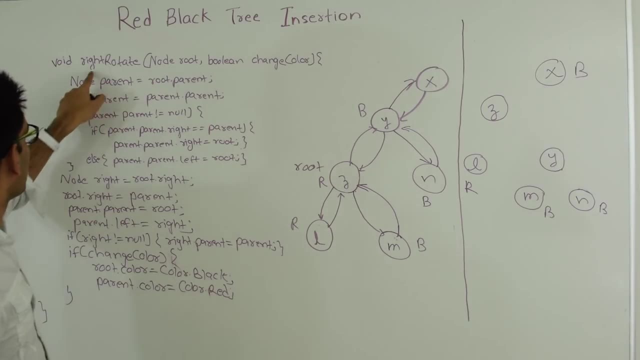 This makes it very easy to get the color of the sibling, because all you have to do is go to the parent, get its other child and get its color. So first let's look at the code for right rotate. It takes in the root around which the rotation is happening. 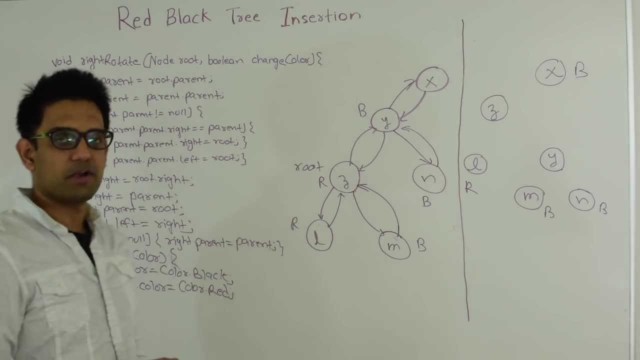 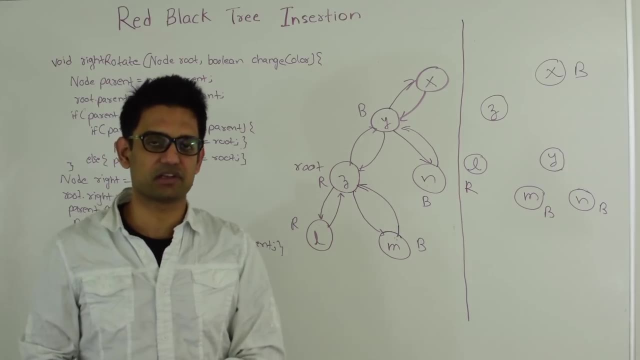 and change color. Let's first talk about change color. So we are doing right rotation in two situations. One is left- left, in which case we are doing one right rotation, and in that situation we are changing the color. So the path change color is. 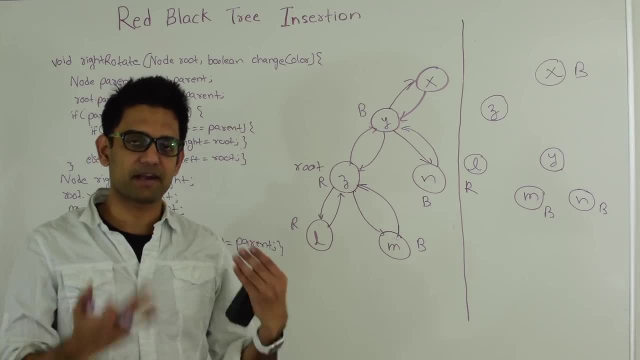 as true In other situation. if we have left right condition, then we do a right rotation in which we do not change color, followed by left rotation in which we do change color. So if we do not want to change the color, we send it as false. 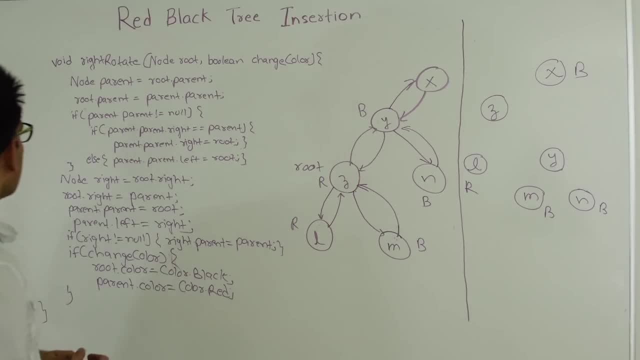 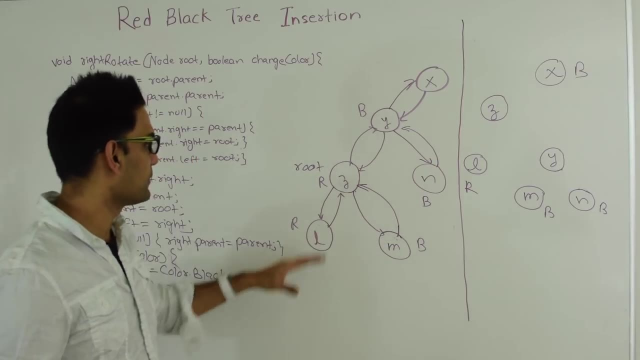 and if we want to change the color, we send it as true. Now let's apply this code on this tree here. Let's assume there are more parts to the tree, but these are the relevant nodes. And also, to avoid the mess, let's update the links here. 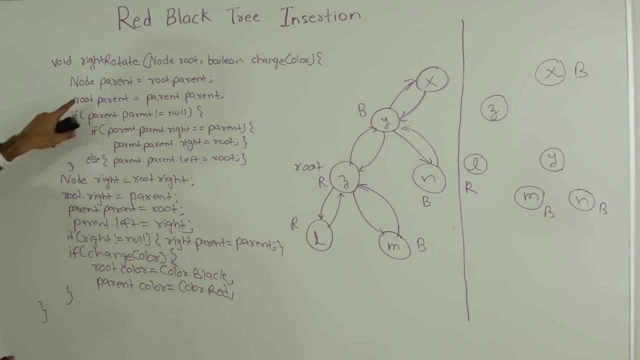 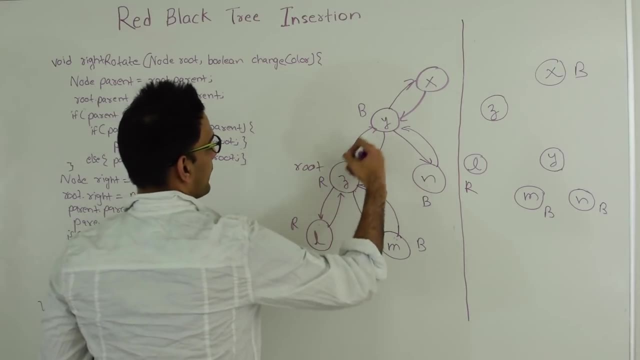 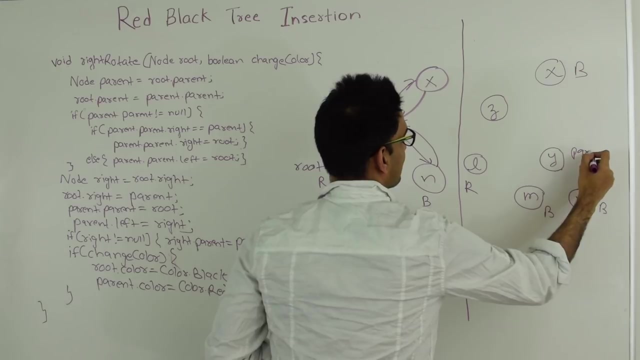 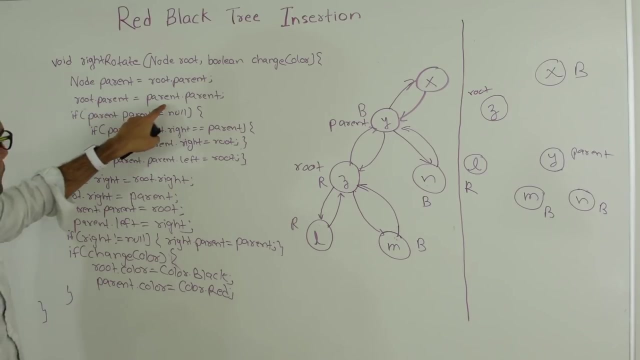 and remove the link from this tree. So node parent, so root is z. node parent is equal to root dot parent. So this guy's parent is y, so this is parent, this is parent and this is root. Then we are going to say root dot parent is equal to parent dot parent. 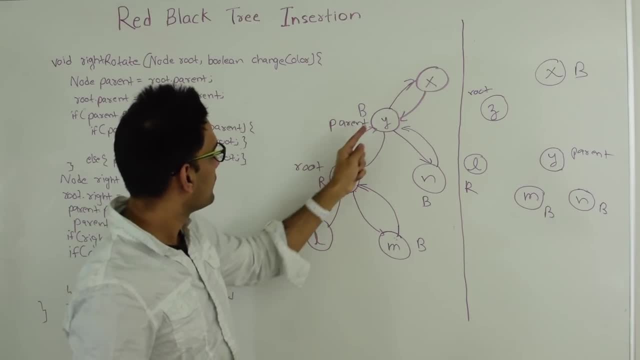 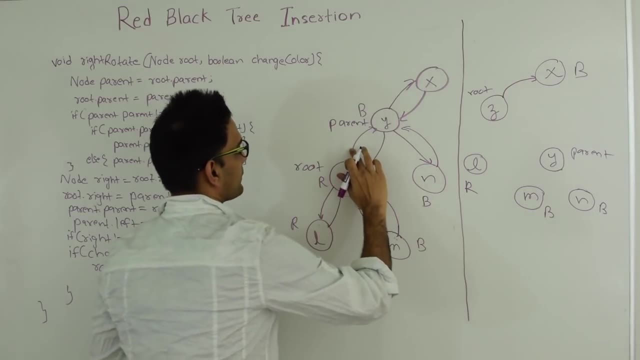 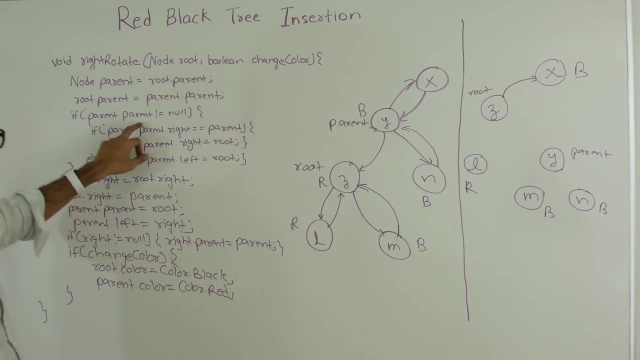 So we are going to change this link from here to point to parent's parent, so x. So what we are saying is establish this link here. So we are going to remove this from here and establish the link from z to x. Then, if parent, parent is not null, 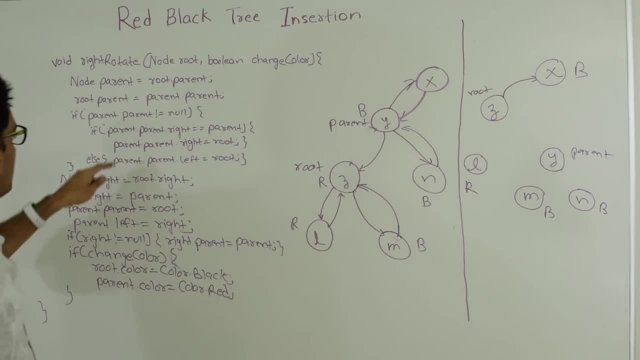 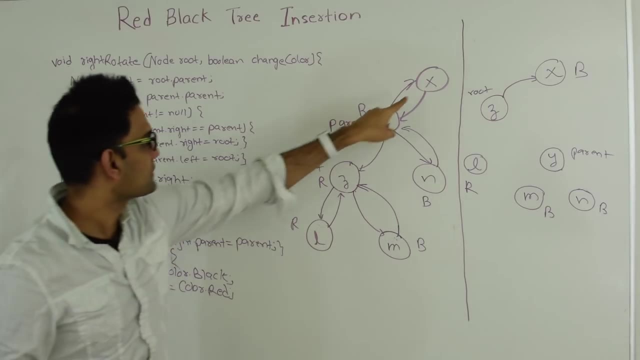 so x is parent's parent and it is not null. then we check: was y the left child of x or right child of x? So y was the left child of x. so it will not go into this if condition parent dot, parent right is equal to parent. 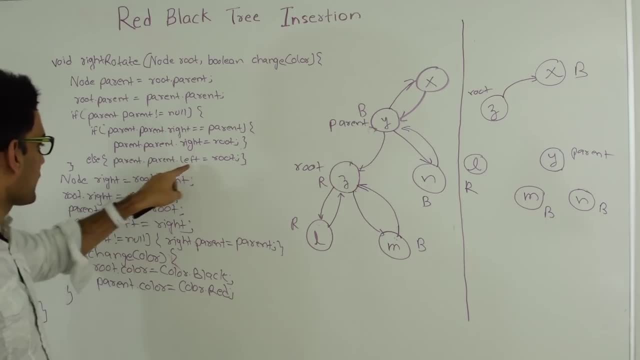 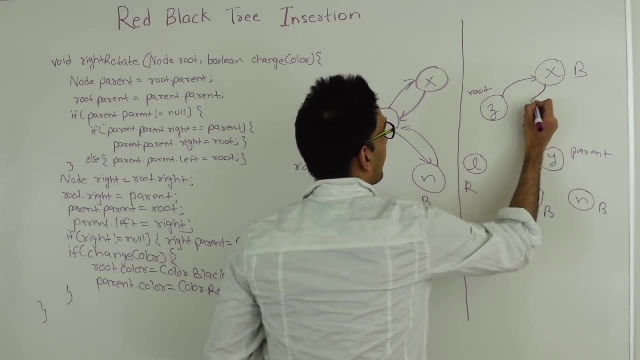 so it will go into this else condition. So what we are going to do is parent dot parent dot. left is equal to root. So parent dot parent is x and its left will point to root, which is z. So basically, we remove this connection from here and establish it there. 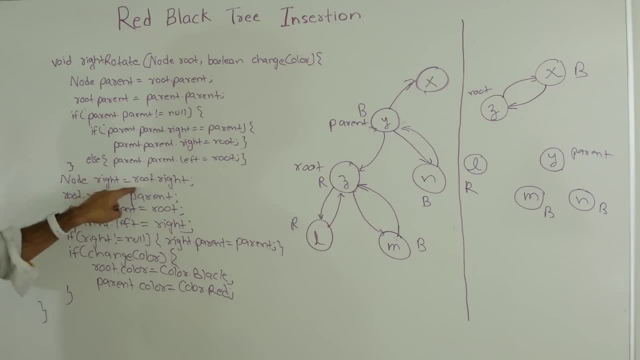 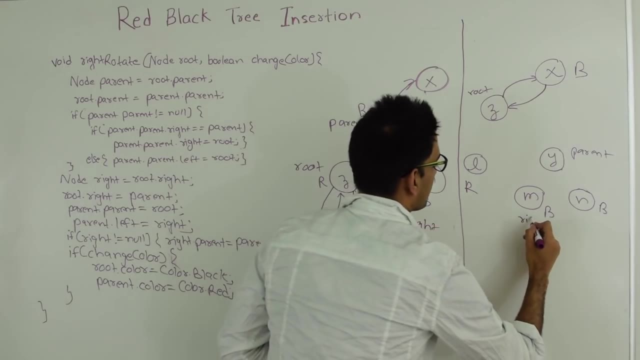 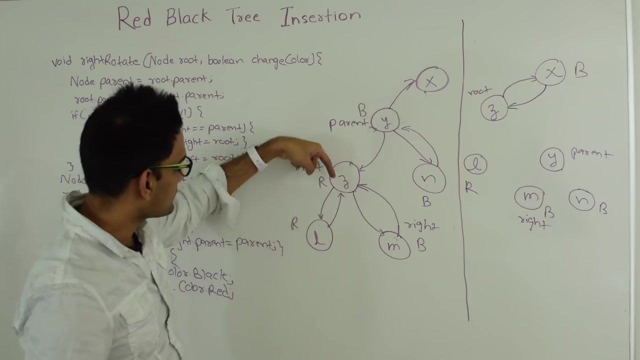 Then we say: node right is equal to root dot right. So we are going to: this becomes our right and this is our right Now. root dot right is equal to parent. So what I am saying is z's right right now is m. So instead of that, z's right will now become parent. 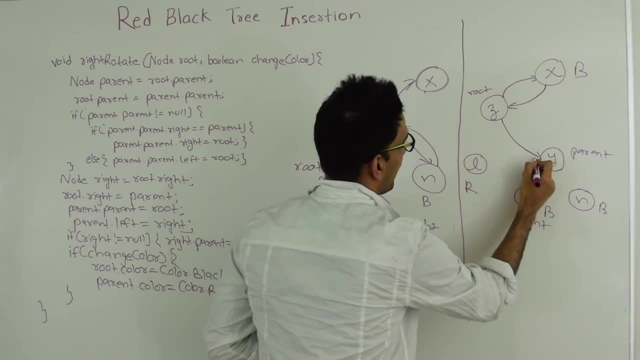 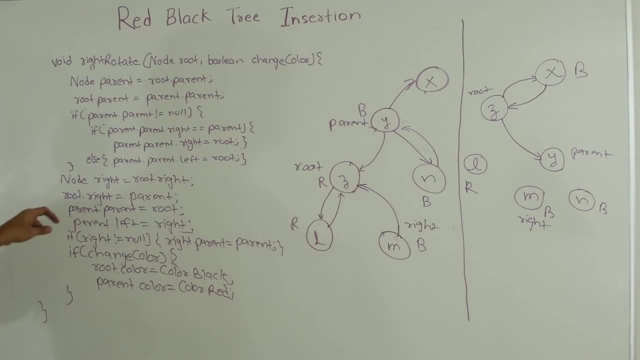 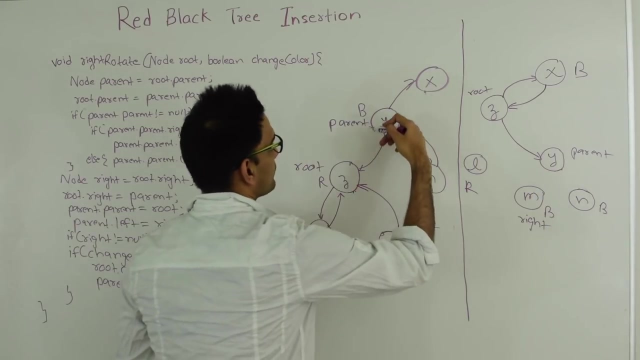 So in this structure here z's right will become parent, which was y, And let's remove that connection from here. Then parent dot parent is equal to root. So this guy is parent And y is parent. It's parent is now pointing to x. 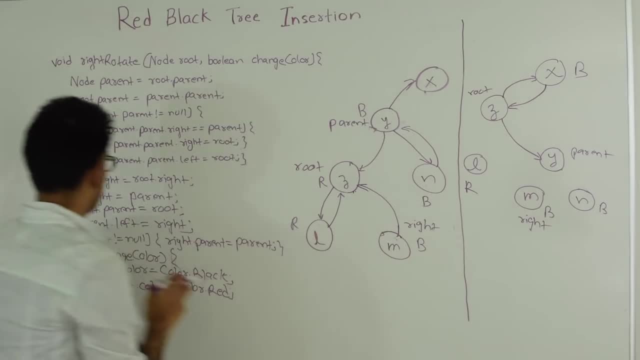 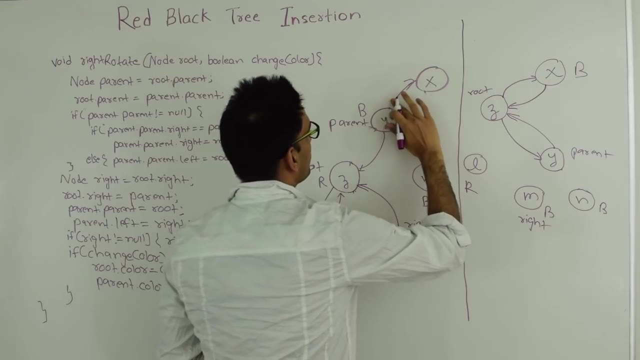 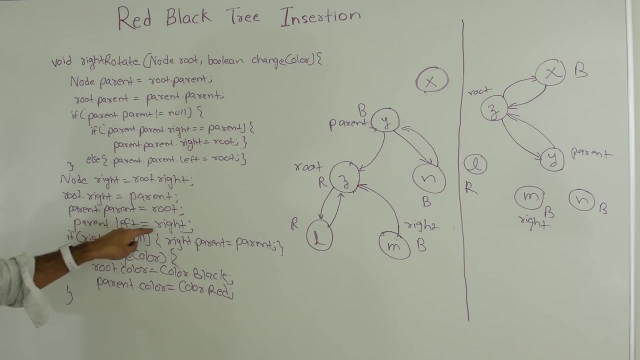 But z is the new parent of y, So we are going to change that and parent dot parent becomes root, So y's parent will now become root, So z. So we remove it from there and add it here. Then parent dot left is equal to right. 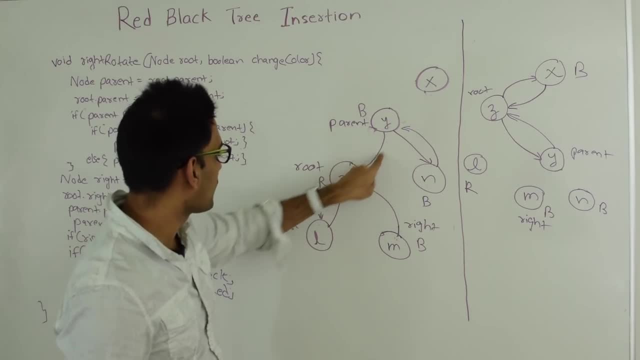 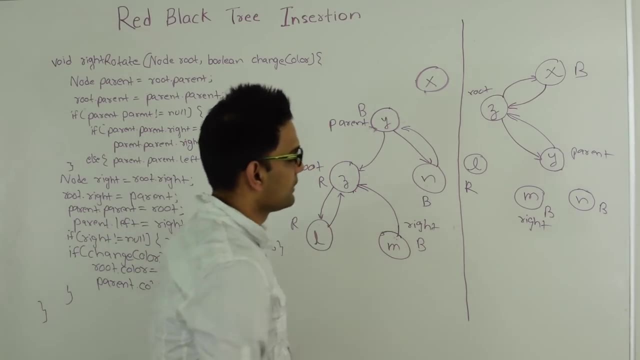 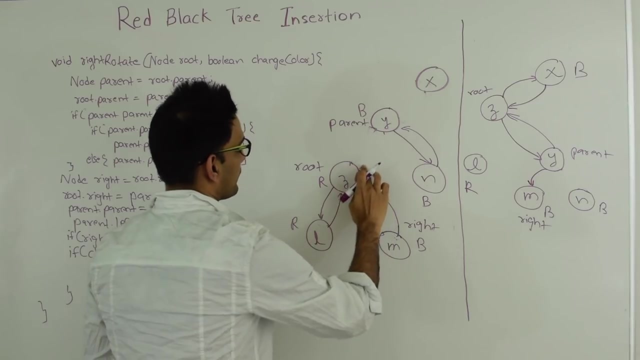 So parent's left right now is pointing to z, But it shouldn't be pointing to z. It should be pointing to m. So right is m. So this guy points to this guy and we remove this connection from here. So y's left now points to m. 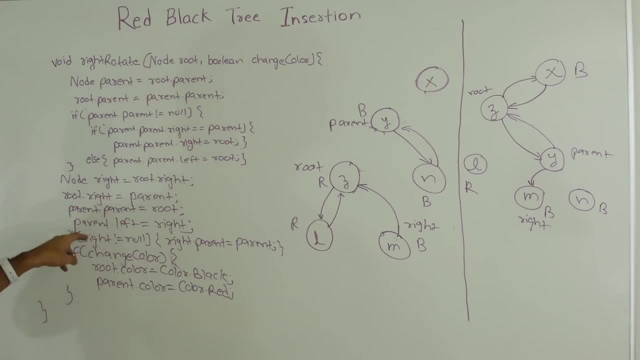 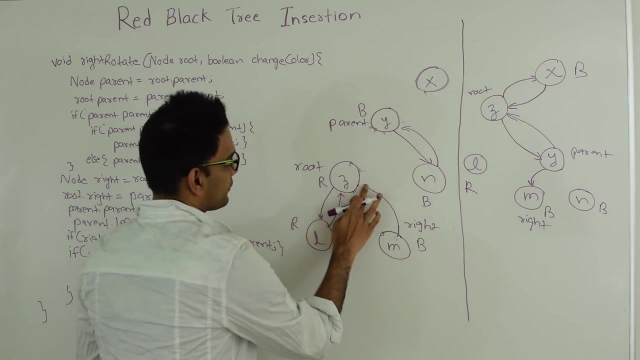 And if parent dot left is right, So parent dot left is right. And if right was not null- It is not null in this situation It's m- Then right's parent will become parent. So right now right's parent is z, So we will break that connection. 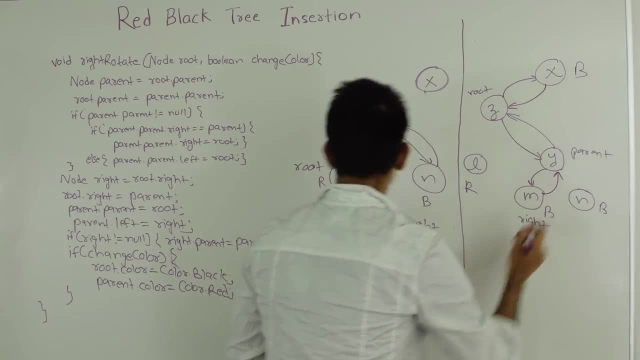 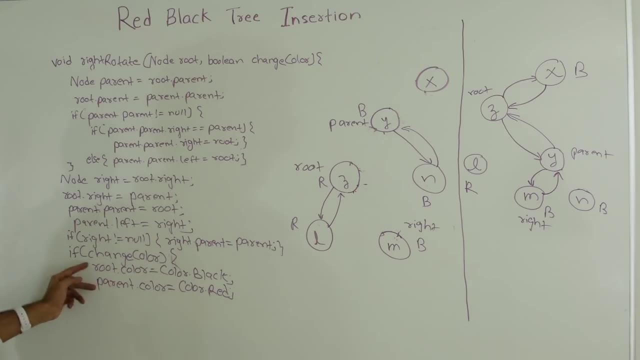 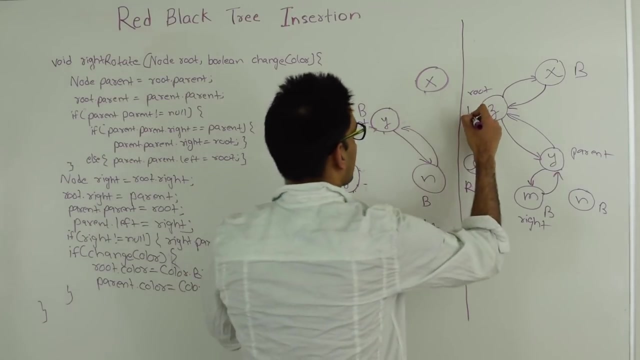 and establish this connection. After that, if change color is true, So change color is true in this situation. So we are going to flip the color of root and parent. So before the move, this guy was red and this guy was black. Now this guy will become black. 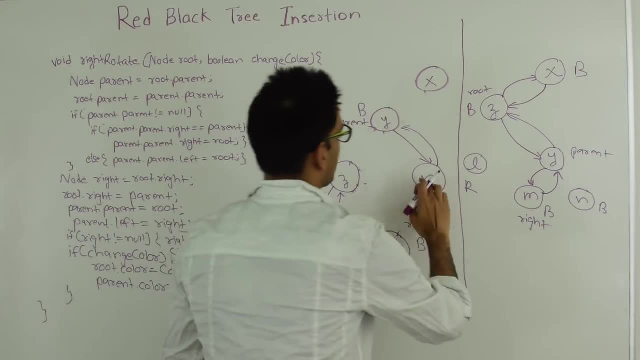 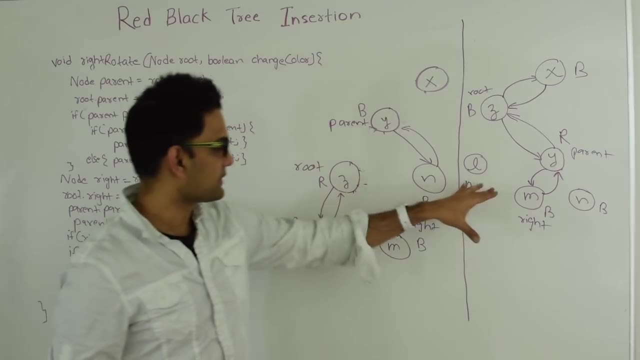 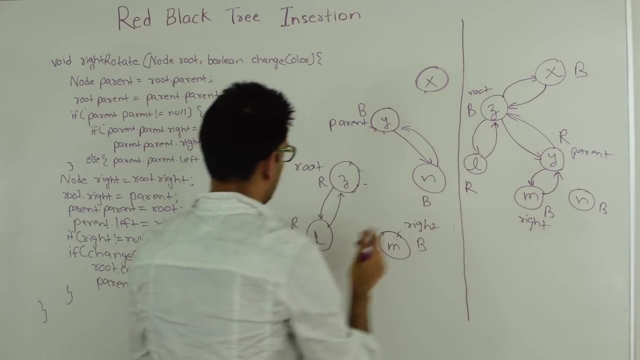 Because root dot color is black and parent dot color, which is y, will become red. So we flipped their colors And this is it, So rest of the connection stay as it is. So l continues to be the left child of z, So we remove this from here. 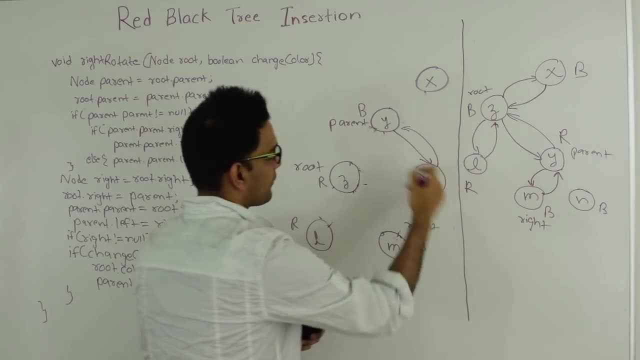 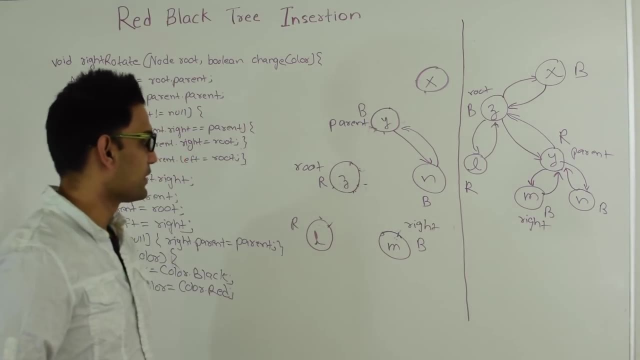 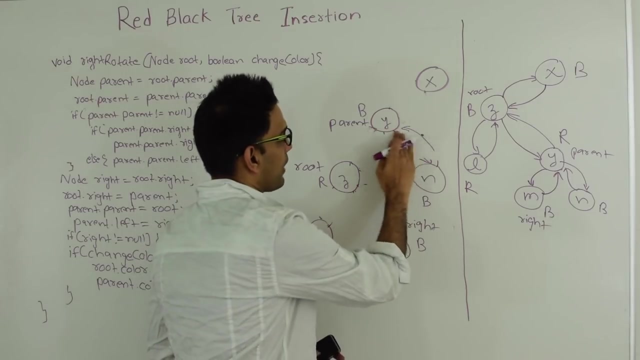 And n continues to be the right child of y, So hopefully this helps you understand how the rotation happened in this case And, as you can see, this rotation can happen in all of one time. So next let's look at the remaining code for red black tree. 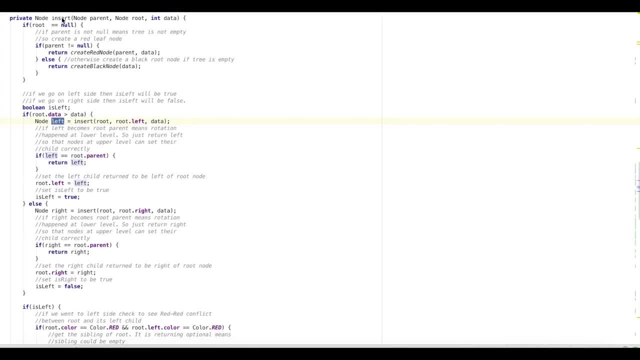 Rotation is a mirror image of right rotation, So we are not going to look at that code. Let's look at the main insert function. It takes in the parent, It takes in the root And it takes in the data that needs to be inserted. 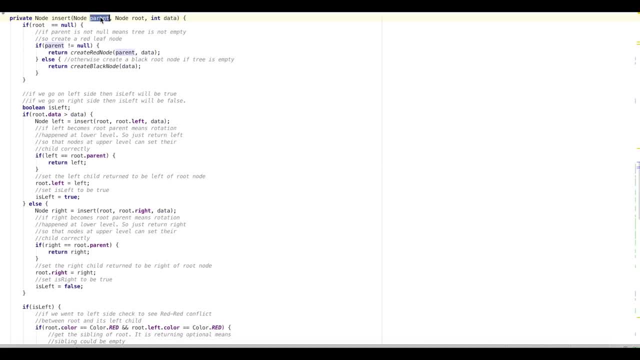 We need parent during insertion because we are trying to establish that relationship from root to its parent. If root is null, it means that we have walked all the way till the leaf. If parent is not null, it means that the tree was not empty. So we create one red node. 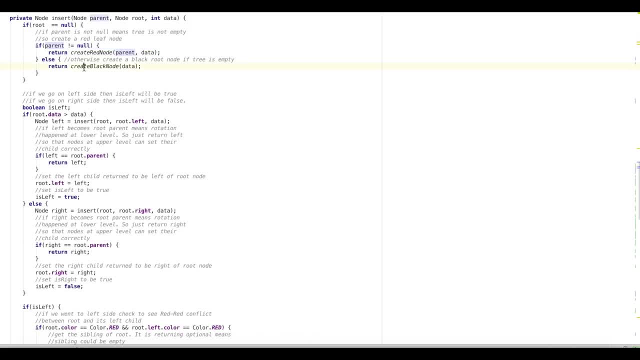 And if the parent is null, it means that the tree was empty. So we create one black root node. This isLeft is going to tell us that if we moved in the left direction or right direction, If rootData is greater than data, then we are going to call insert recursively. 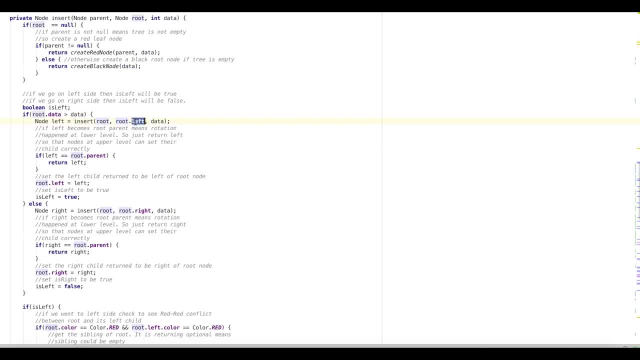 This time the new parent will be root, And then we are going to pass rootLeft as the new root of the left subtree And then we are going to pass the data that needs to be inserted, And then we get a left result And then we get a left node. 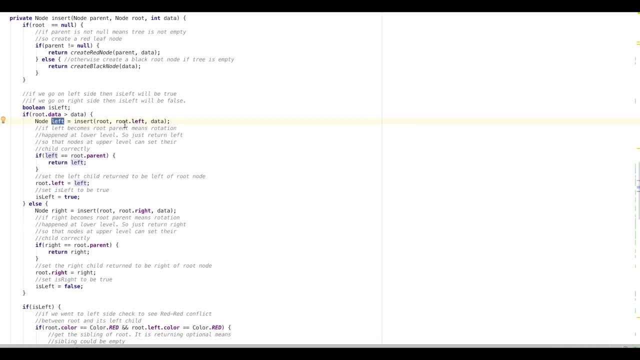 back from the insert. This left node could be the same as the rootleft as we passed in, Or this left node could be the newly created left node, Or this left node could be another node which could have been the new root of that left subtree. 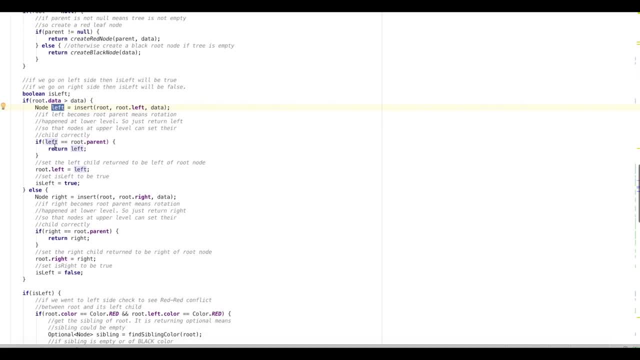 which would happen in the case of rotation, If left is equal to root parent. what this means is that rotation happened on the left side and root is no longer the parent of left. In fact, left is the parent of root. In that case, we want to return left. 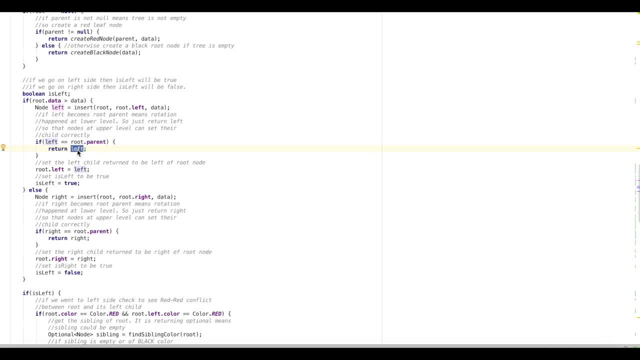 so that the level above us can set their left or right child correctly. Hopefully this F condition makes sense. Otherwise, if that did not happen, then we just say rootLeft is equal to rootLeft. So we are setting the root's left pointer to the left, which came back. 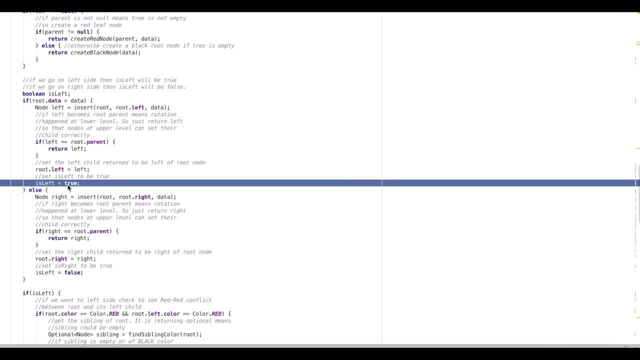 from the insert recursive function And then we are going to set: isLeft is true because we went on the left side, And then we have a similar logic on the right side and in the end we said isLeft to be false because we moved on the right side. 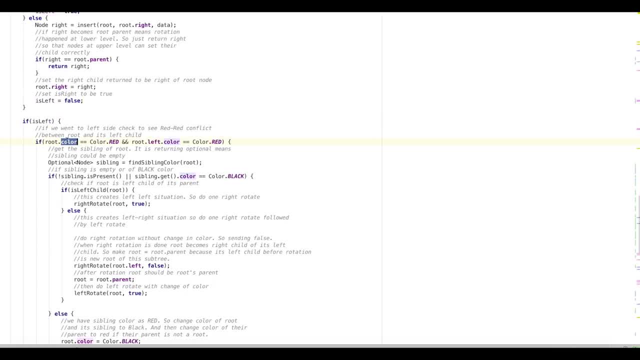 So now, if isLeft is true, it means that we went on the left side- then we are going to check if the color of the root is red and if the left child is also red, it means that we had this red red situation. So what we are going to do is 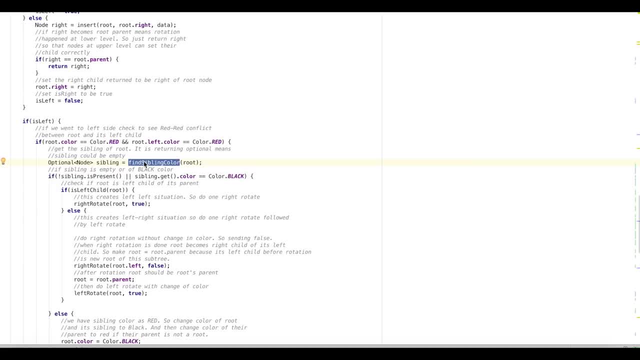 we are going to get the color of the sibling. So this find sibling color. all it does is go to its parent and gets the color of its other child And it is returning optional because this sibling could be absent. So if sibling is not present, 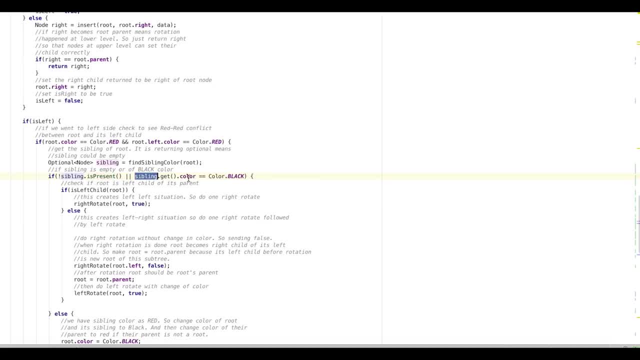 so if present is false, or if it is present and the color of its sibling is black, it means that we have a rotation scenario, And what rotation to do is dependent on left, right or left left or right left or right right situation. So isLeft child root. 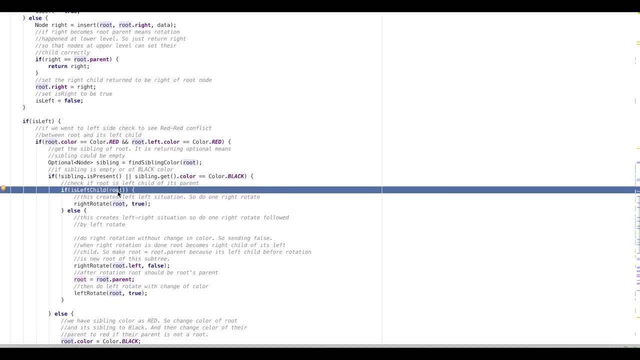 so are we are checking: is the root a left child of its parent? If it is, it means that we have a left left situation, Because isLeft is true, it means that the child at which we are getting a conflict is a left child. and since isLeft child is also true, 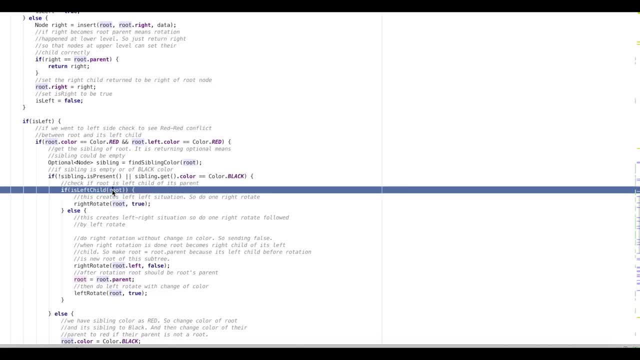 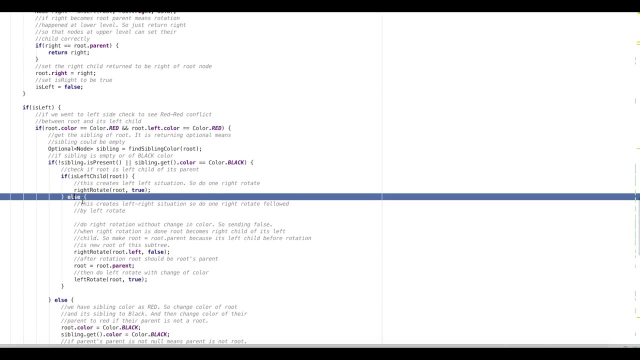 it means that root is a left child of its parent. we have left left situation. in that case, we do one right rotation and we already looked at the code for the right rotation and we are passing through because we are changing the color after the rotation Else. if that did not happen, 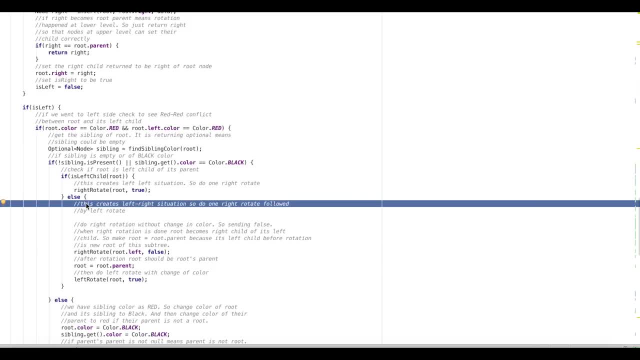 it means that we have a left right situation. So the child with which I am having a conflict is my left child, but the root itself is a right child of its parent, So we have a left right situation. so when we have a left right situation, 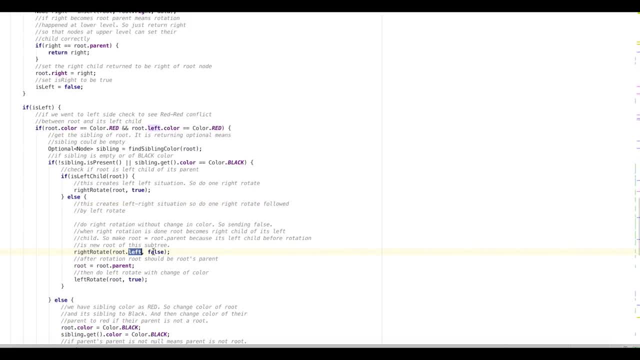 we do a right rotate at the root's left and we pass false because we don't want any coloring to change. and then this root left will be the new root after the rotation of this subtree and it will also be the parent of the current root. so we will set root is equal to root's parent. 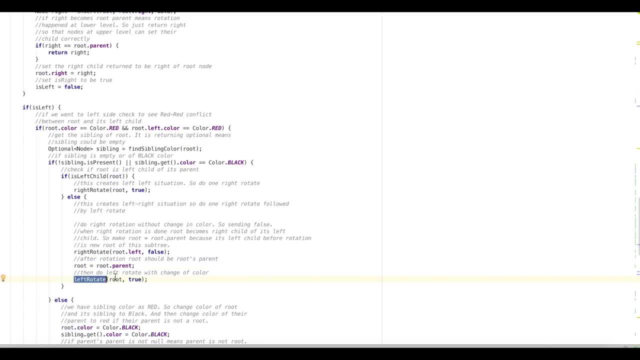 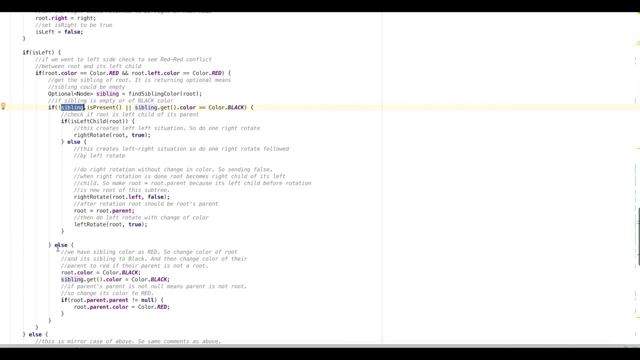 and then we are going to do a left rotate at root and passing through, which means that change the color during this rotation, else, if the color, if we come to this, else it means that the color of your sibling is red. in that case we say root color. 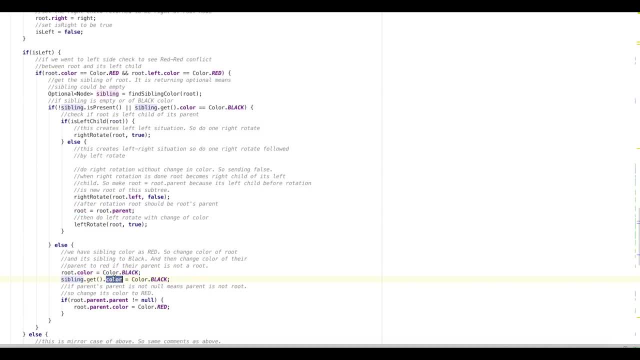 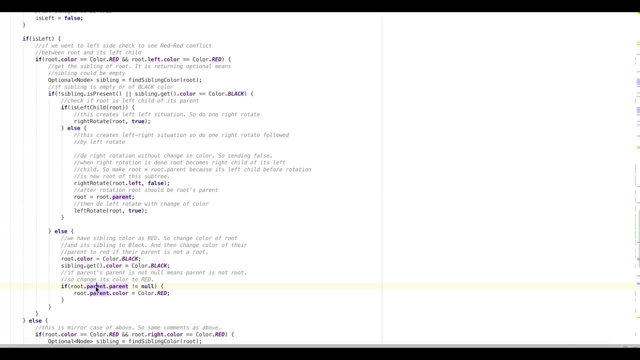 so we change the color of root to be black, we change the color of its sibling to be black and then we check if that parent is not root. to do that, we check. if parent's parent is not null, it means that parent is not root. so we change its color to be red. 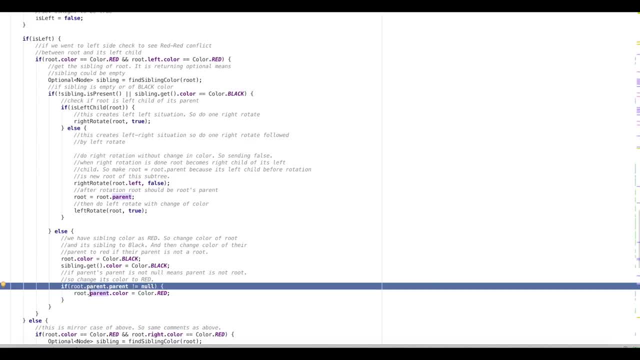 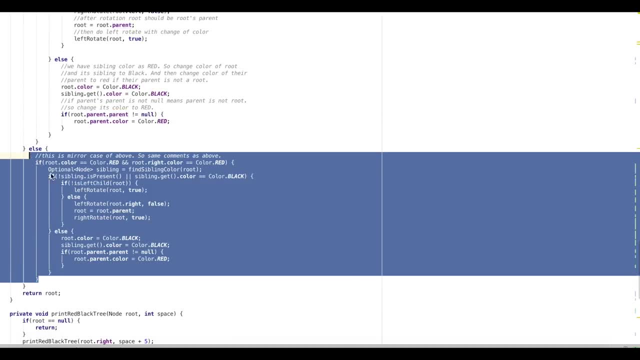 and if it was root, then we leave its color as black. and similarly, if it did not go into the left side, then we would have gone onto the right side and right side would have exact opposite mirror case. so right side would either have a right, right situation. 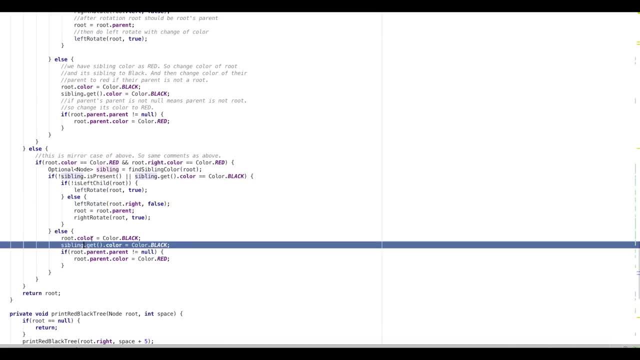 or it would have a right left situation, or it will have. the sibling's color will be red, in which case we will do some recoloring and finally we return this root and so when it comes back from the recursion, the level above, you will set up the. 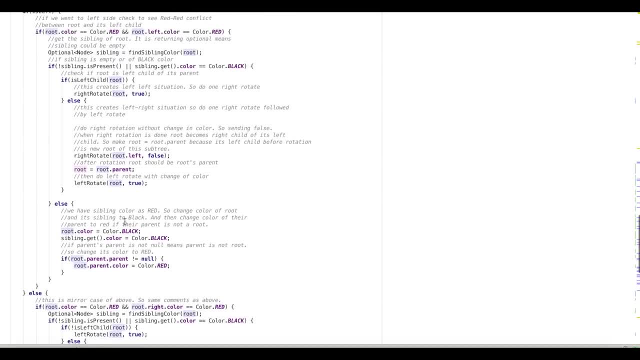 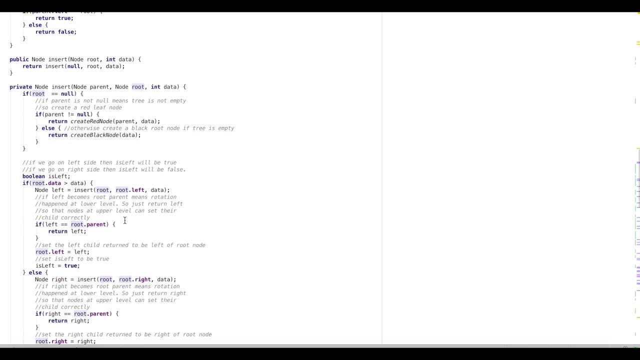 value of its left or right child correctly. so hopefully this gives you some idea on how this insert is happening. so this is all I have to talk about. red black tree again. the runtime complexity for insert, search and delete is off. login time. so guys like this video.